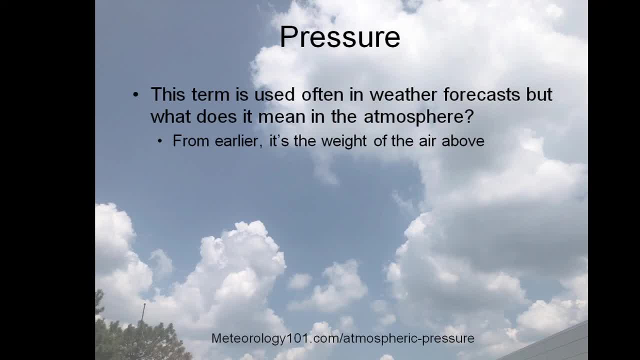 start experiencing pain. so that's when people say their joints start hurting when uh weather's coming in. so how about weather? does how does that pressure interact with the weather? high pressure is usually 19 weather. low pressure associated with stormy weather. so we talked about before, was uh cold. 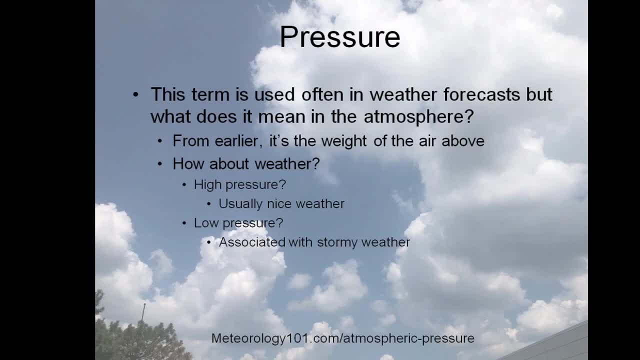 air doesn't hold as much moisture. cold air is more dense than warm air, so cold air suppresses any cloud development or any weather, and that's why you have just a nicer weather. typically, you'll get um some cumuliform clouds, just some cumulus. fair weather, cumulus pop up. 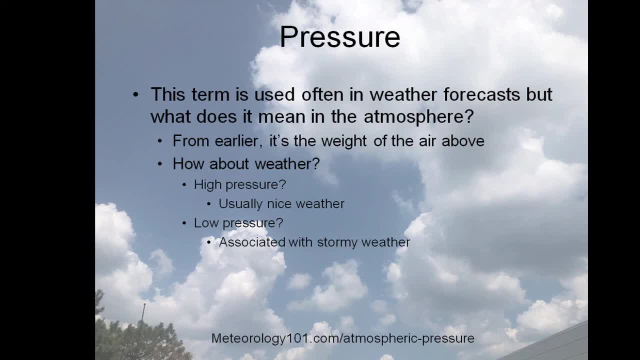 or around those high pressure systems. as the high pressure system comes in, that causes the lift and pushes that low pressure up. so now that moisture is being lifted and then you'll get that stormy weather like we talked about with the low pressure system, a cold front passage, and then 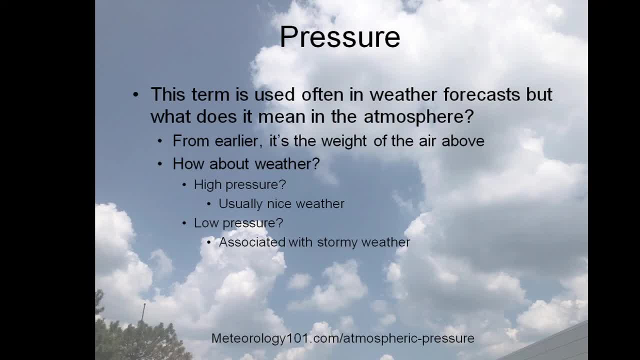 there's, uh, three things you need for stormy weather. it's moisture, instability and lift. and then air tea isOME. you have to pull all the air up you made or remove it when some air is air. tail yourself did k air noi, welcome Jesús. pushing that warm air loft and where it wants to be. and then the moisture: cooling the air. 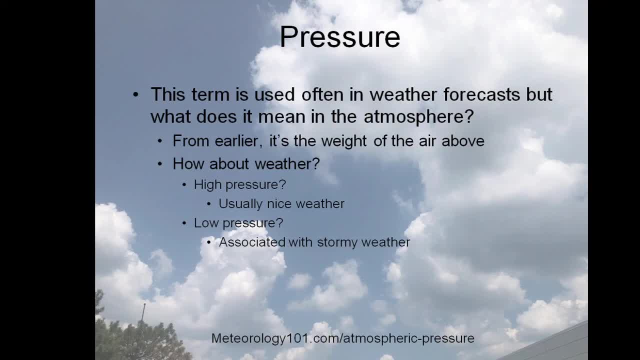 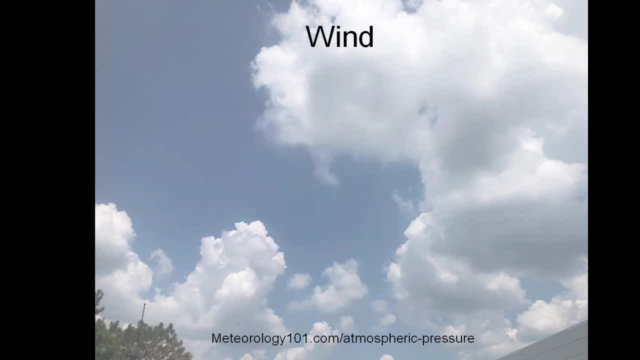 expands, cools, condenses, creates those clouds, and then the water droplets collide, get bigger and they want to fall to the ground. so, sticking on topic with the pressure in the air, air pressure and wind- another element we deal with on a regular basis is wind. but why does? 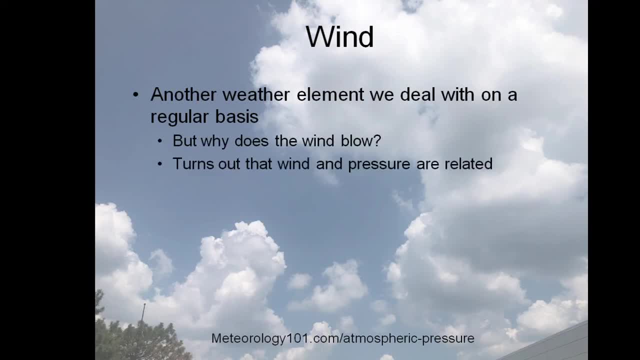 the wind blow. well, it turns out, wind and pressure are related. so the, in fact the wind blows due to horizontal differences in pressure. so if you have an area of high pressure, so if there's high pressure over one part of the of the country, low pressure over the other, 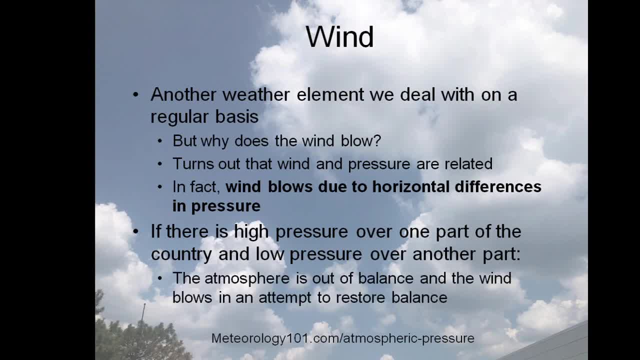 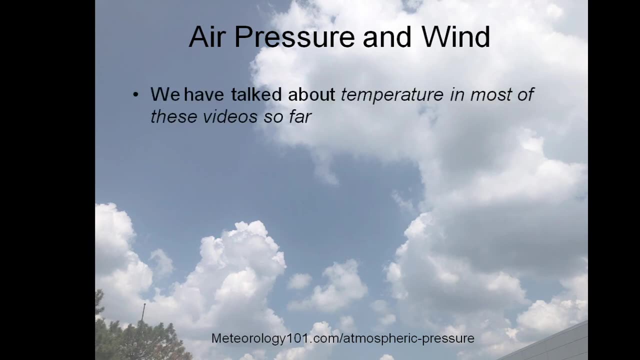 part of the country, then that's when the atmosphere is out of balance and the wind blows to attempt to restore that balance. so high pressure blowing into low pressure to restore that balance and that's what you're feeling as the wind blows. all right, we talked about temperature and most of the video so far. temperature is a major player. 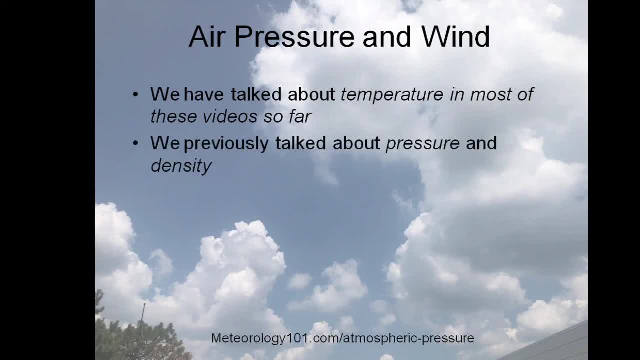 in atmospheric weather. we've mentioned that over and over and we also talked about pressure and density. so the higher the density, the higher the pressure, so the atmosphere, these variables are related, such that a change in one will cause changes in the other. so there is a balance there. 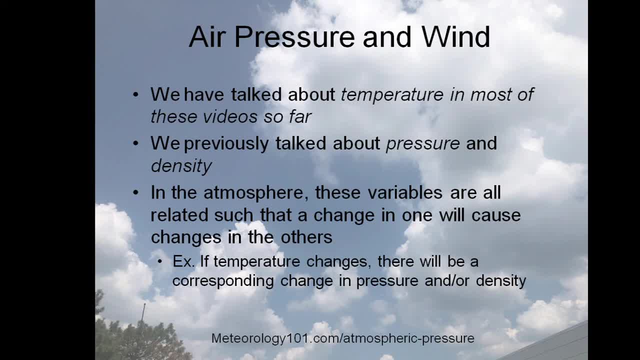 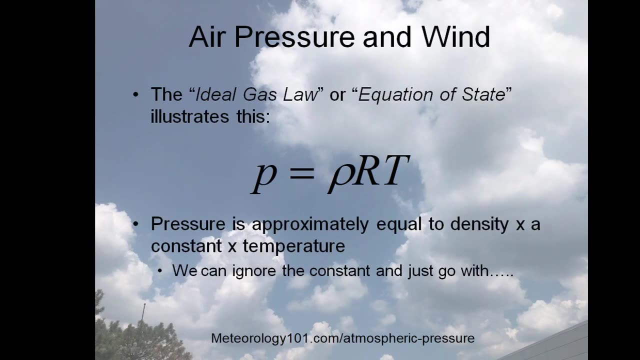 for example, if temperature changes, there will be a corresponding change in pressure and or density. so warm air is lighter than cold air. so if the air warms up it will be less dense and want to rise, creating lower pressure. the ideal gas law or equation of state illustrates this. so pressure 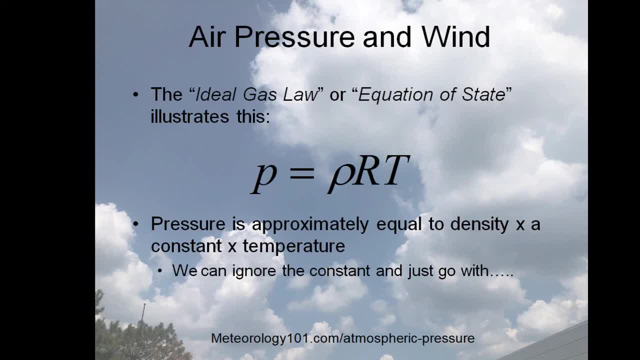 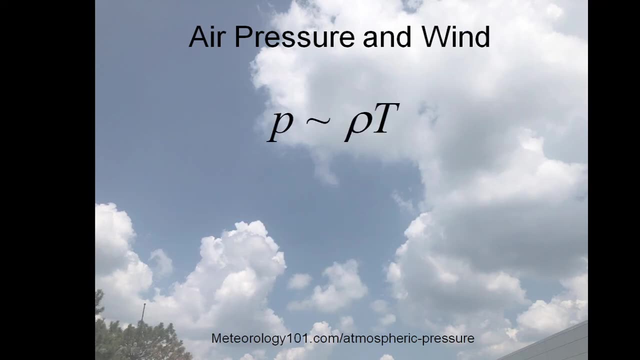 equals as approximate. equal to density times a constant times temperature, and. but we can ignore the constant and just go with the change in density and temperature. so if the pressure doesn't change, an increase in temperature results in a density, a decrease in density. so warmer is less dense, therefore it rises. a decrease in temperature results in increase in density is. 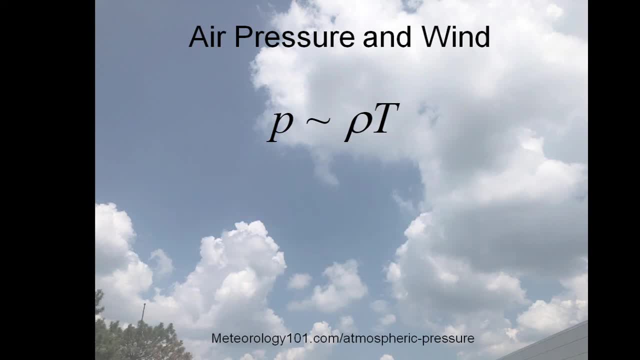 cold air is more dense wants to sink. so if the temperature doesn't change, an increase in pressure results in an increase in density. decrease in pressure results in a decrease in density, so it almost seems backwards. but the an increase in pressure. if you're pushing down on the atmosphere, you're pushing all the. 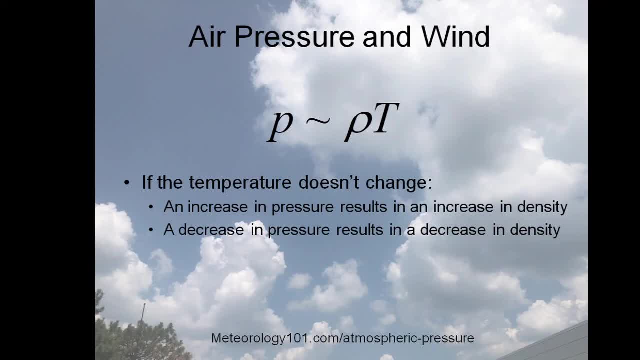 molecules to the surface. that's creating a higher pressure and a higher density. so if the air temperature drops then the higher heights of the heights of that air column would drop and compress, all that make it become more dense and it'll be a higher pressure. so at the same temperature, air at a higher 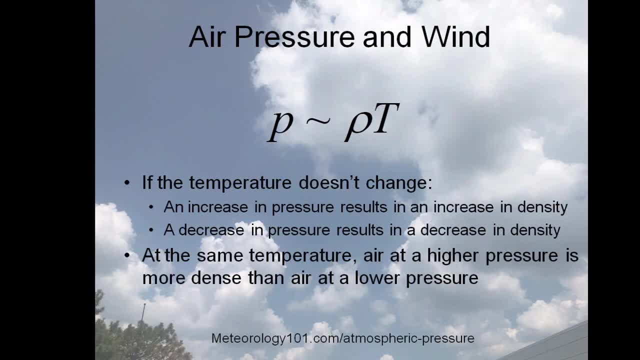 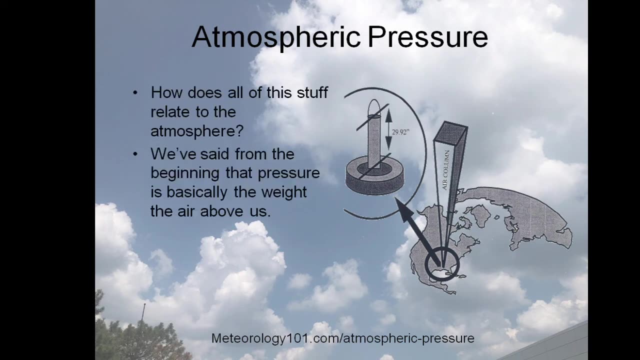 pressure is more dense than air at a lower pressure, like it's just that you're compacting those, those molecules, to create one more dense air parcel. so atmospheric pressure: how does it relate to the atmosphere? we've said from the beginning that pressure is basically weight of the air above us. 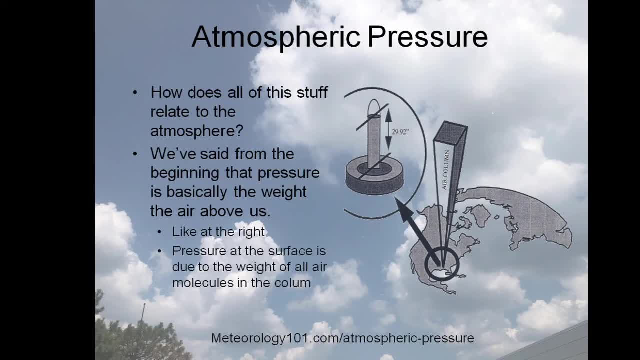 like we show at the right, that column of air. if you weighed that column of air, that would actually weigh about the weight of a large elephant. like I said, because of blood pressure you don't feel it. the pressure at the surface is due to all the air molecules in the column. so if you took all the air molecules in that column and 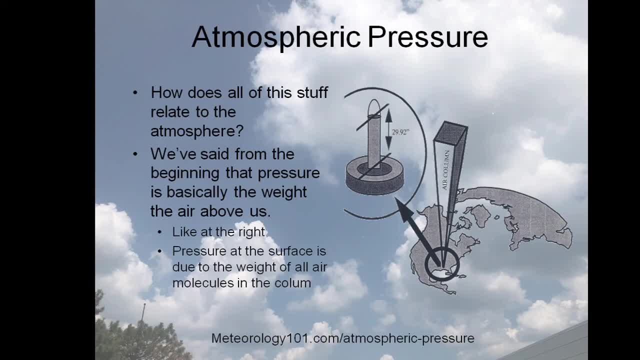 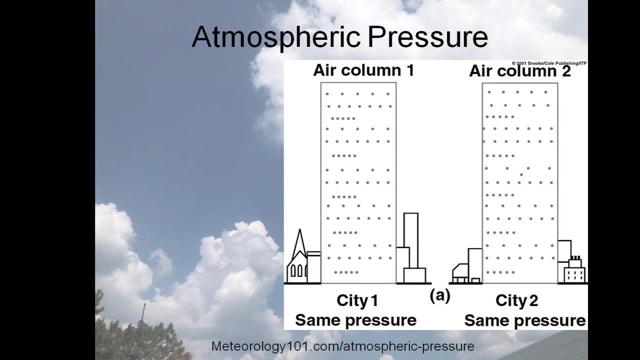 you weighed them. now, if you took all those air molecules and push them down into a lower volume of air, then you'll have a more dense volume of air and that would be higher pressure. okay, with the two cities with the same pressure and two different air columns. 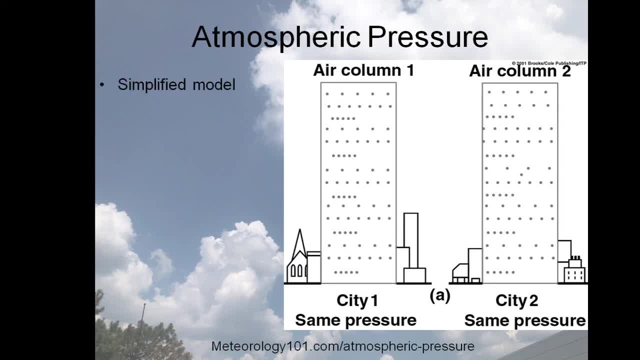 we assume the air can't leave the columns and the air columns have the same number of molecules and are at the same temperature. the pressure at the surface is the same. both cities are equal. so what would happen if we change the temperatures of those cities? well, there's columns of air above those cities. 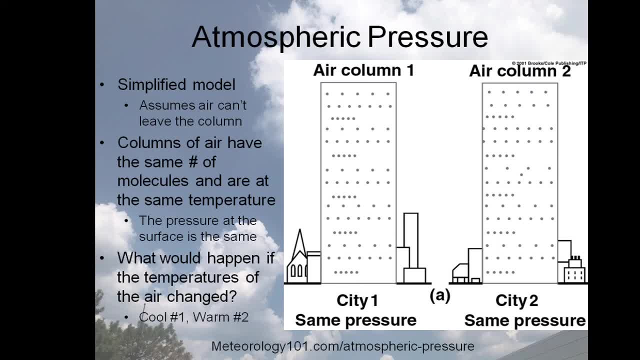 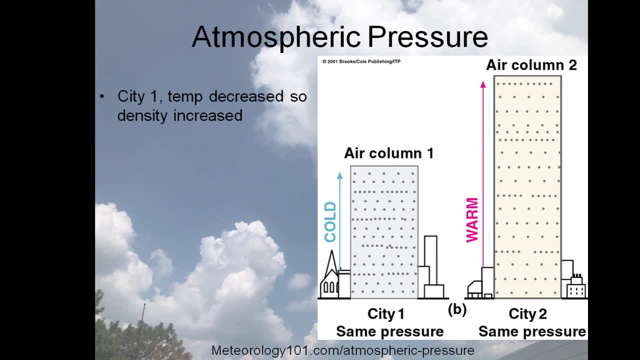 what would happen then if we cooled column number one, warmed column number two, so column number one would actually decrease. the height would decrease, so the density would increase. so the temperatures decrease, the density increases. cold air is more dense than warm air and then city two temperatures increase, causing the density to decrease. 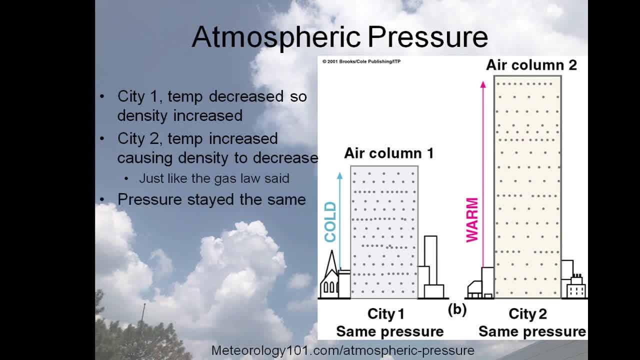 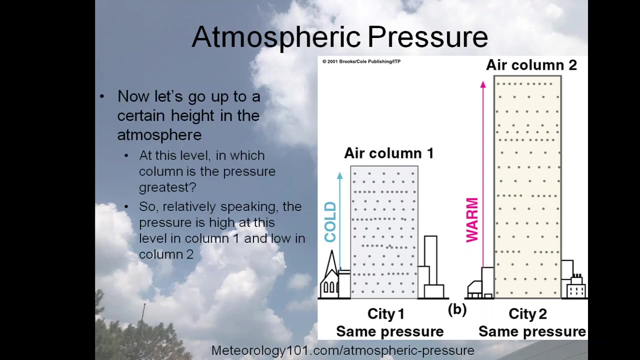 just like the gas law said and put, pressure stayed the same. so the bottom line of this is the shorter column of cold air can exert the same amount of pressure as the taller column of warm air, because the density remains the same, so the pressure remains the same. now, if you go up to the certain height of the atmosphere at this level, in which column is the pressure, 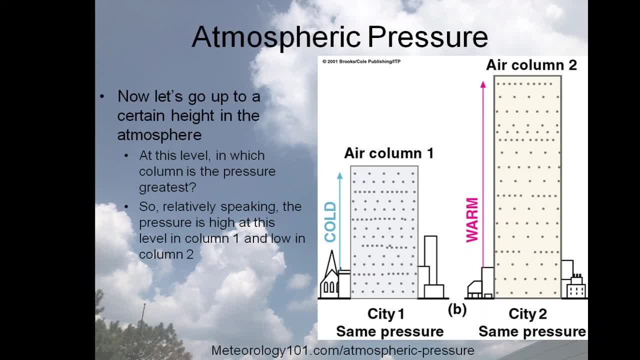 the greatest. so relatively speaking, the pressure is high at this level of column 1 and low at column 2. so if you draw a line across these columns and you have the cold, dense air, you still have higher pressure in the warmer air because you have more, more of an air column above, more air above that level, so you have more. it's more dense, so you 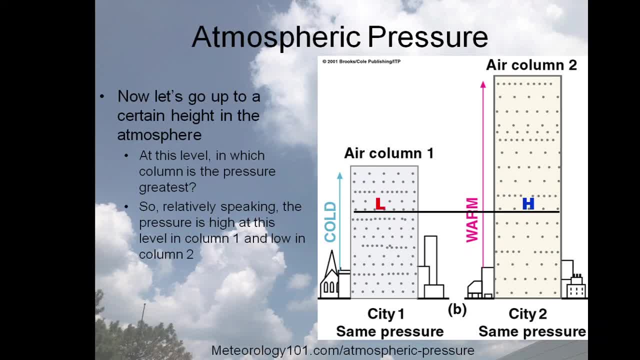 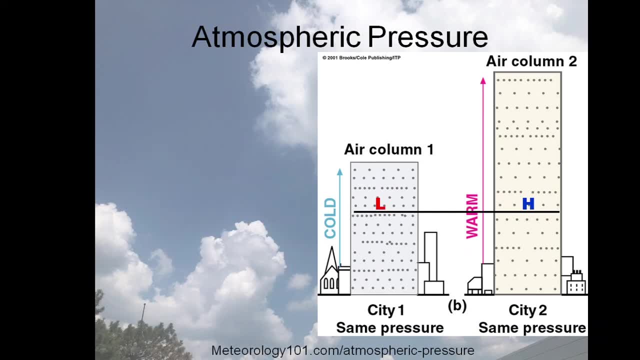 have a higher pressure in the cold air. you're just cutting the top of that cold air column off so you have a lot less density up there, so you have a lower pressure. so the points of this pressure changes more rapidly with height and cold air masses. warm air loft is associated with high pressure aloft and 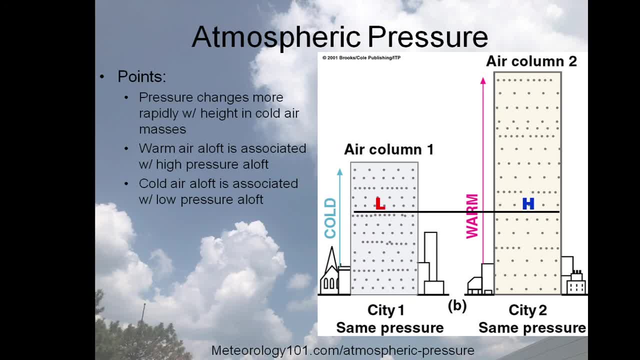 cold air loft is associated with low pressure. aloft it's actually like on a hurricane: you'll have a surface low and it extends to the upper levels. but you actually, if you get up to about the 300 millibar level, you're actually reading a. 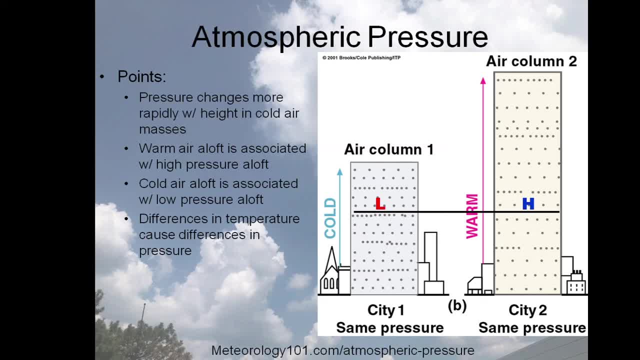 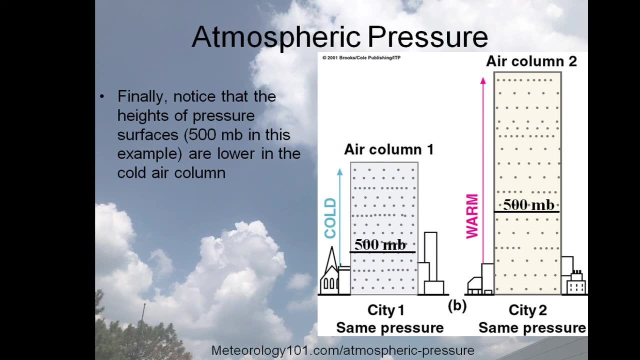 high pressure on the on the constant pressure chart, about 300 millibars, about 30,000 feet. so the difference in temperature causes differences in pressure. and notice that the heights of the column, heights of the pressure surface, is 500 millibar in this example or lower in the cold air column. so if you have a 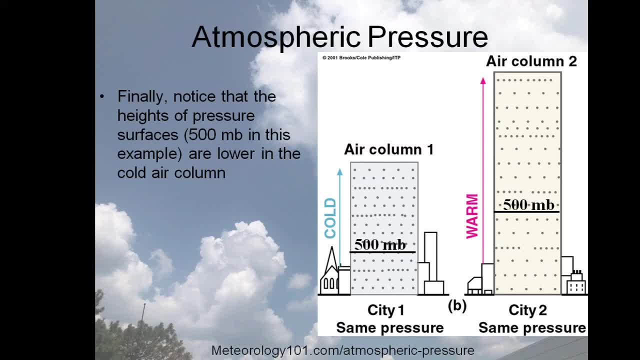 500 millibar level. that pressure is lower in the cold air column than it is the warm air column. so now you have higher heights in the in the warm air to reach your 500 millibar level. that pressure then yeah, it's, warm air is less. 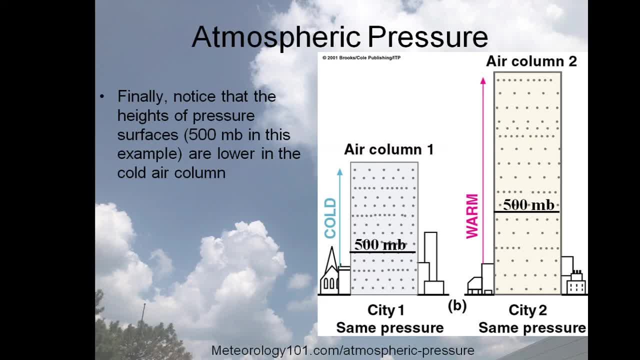 dense, so you have to go to a higher level to reach your 500 millibar level. but if you have a pressure that is higher, you can go to a higher level to reach the 500 millimeter pressure level. so now the air movement is always from high to low. 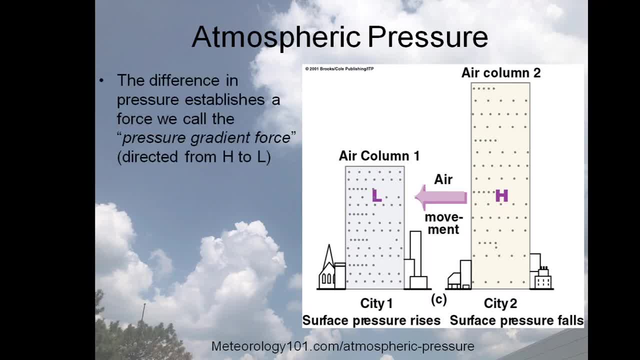 pressure. the difference in the pressure establishes a force that's called pressure gradient force and it's directed from high to low. now if we remove the side barriers of the columns, there will brush them to high to low pressure T in order to equalize things. so now you're taking that there's tubes. 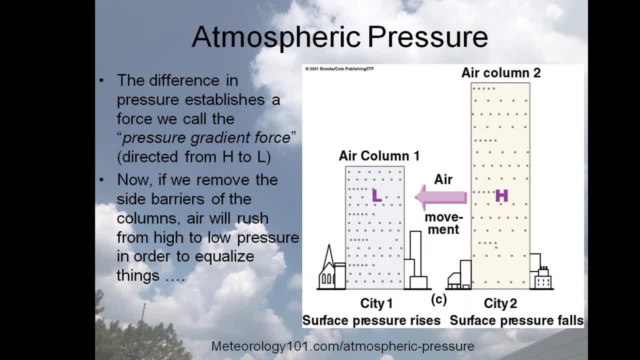 out and just letting that air flow like the atmosphere does, and that's just how you're running air from high to low pressure levels. the high pressure is rushing over to the low pressure, and that's what we're feeling for when the wind blows- and that is wind, so pressures at the surface also. 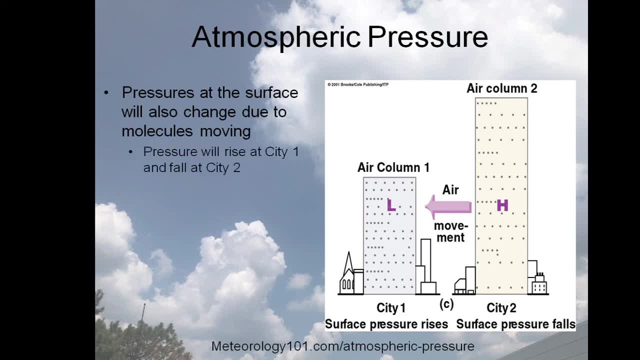 change due to molecules moving. so the pressure will rise at city 1 and fall at city 2. so as they equalize the high pressure blowing toward the low pressure, then that low pressure will start to fill and then the pressure will start to increase and it's taken away from the high pressure. so now the high 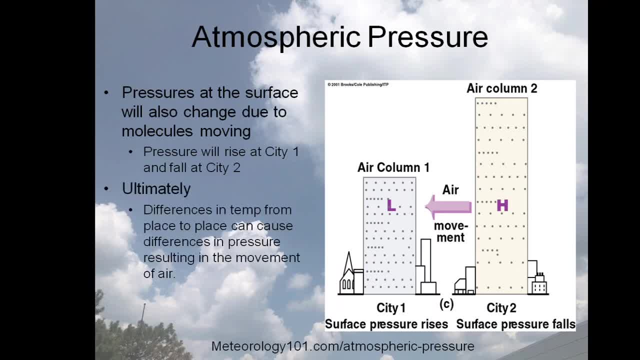 pressure will start to decrease. so ultimately the differences in temperature place to place can cause differences in pressure result and then the movement of air. so we have a cold city in a warm city. the cold air is going to blow toward this higher pressure typically, so it's going to blow. 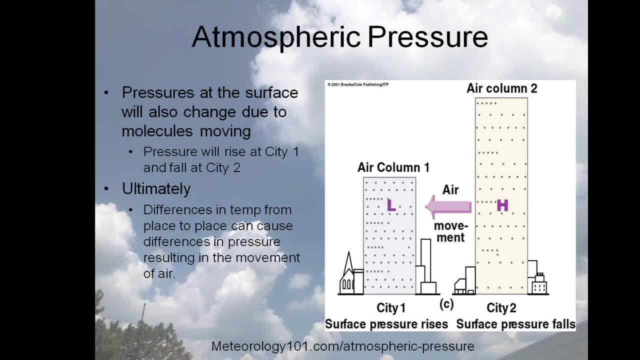 toward the, toward the warm air. now in the upper levels, like we said, the higher, the higher heights, then that's where you, if you're at the 500 millibar level, you have more density, more molecules above you in the low pressure area. so it is a higher pressure at the higher height. so you have to then that. 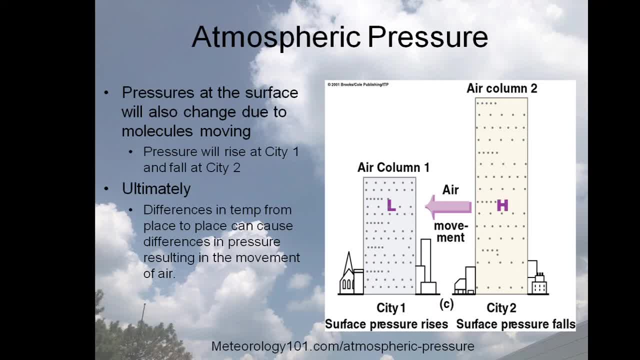 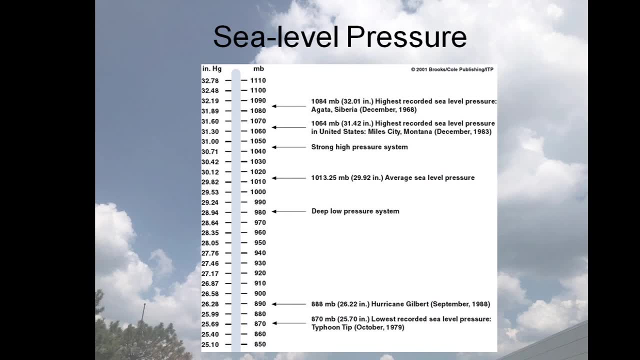 would push over to the. basically, the warm air is pushing to the cold air because it's? because it's simply of the density and the pressure difference. okay, so sea level pressure. the standard sea level average sea level pressure is 1013.25 millibars. 29.92 inches of mercury. that. 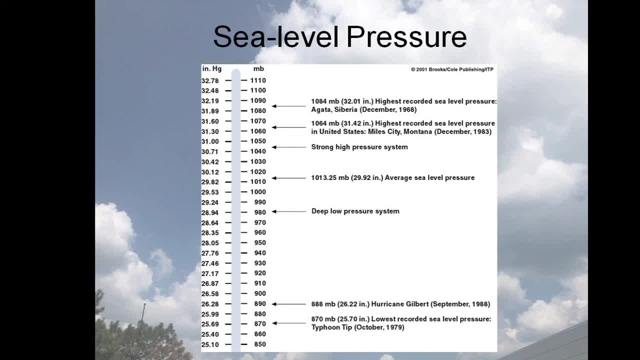 is the average pressure. so if you look at this chart, we got a thousand eighty four millibars, 32.01 inches, the highest recorded sea level pressure and that was in Siberia in 1968. that was Siberia. I remember when I was a kid they always talked about Siberia. he 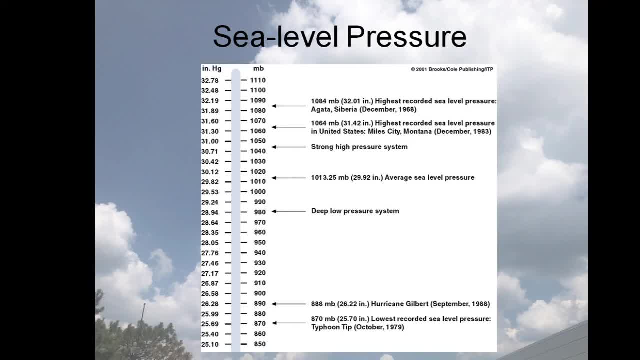 always thought about tons of snow and freezing all the time. then 1064 millibars, 31.42- the highest recorded sea level pressure in the United States, Miles City, Montana, 1983, and right around the 1045- 1043 mark is a strong 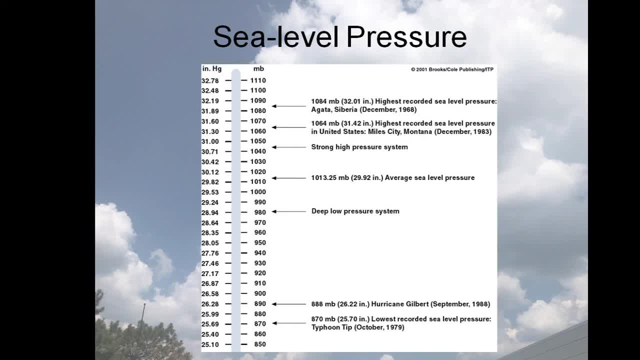 high pressure system 1043 millibars. so if you're getting up in the 1050 millibar you have a real strong like an Arctic air mass. that's gonna be pretty much an Arctic air mass. like we see with the polar vortex is a cold air breaks. 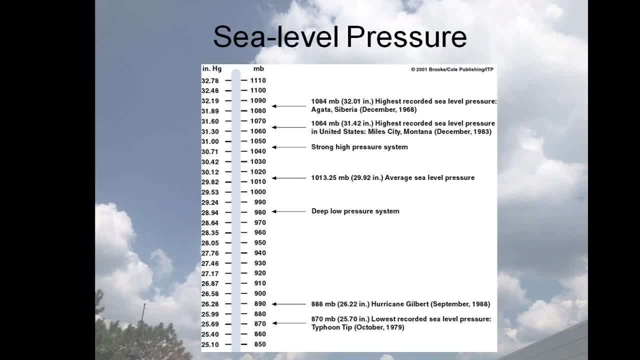 out of the Arctic. that's what you're gonna see for those pressures and the high, the high pressure as it moves south. alright, so around the 980 millibars, that is your deep low pressure system. that's what you're gonna see around the United States- pretty strong low pressure system. moving to the United States to 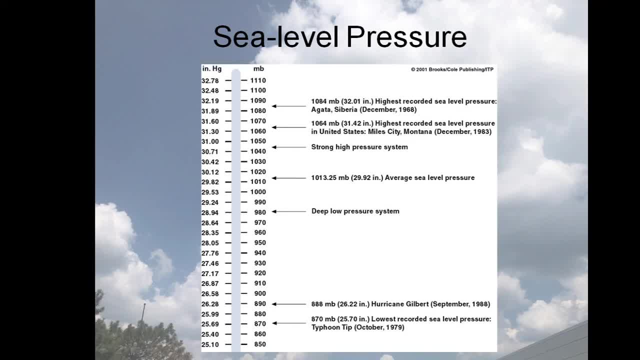 be a, basically something that started down at the Gulf states, low pressure developed and before it moved north that would actually, as it moves north, you would see that system deep and if it had jet support and sucking all that air mass out of that low pressure system and causing that low to deepen, you get to a 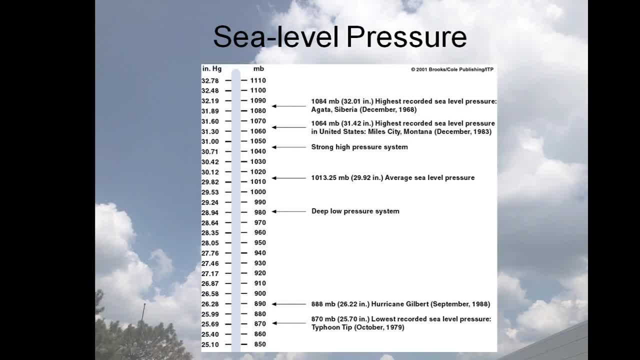 980 millibar level, you got a pretty strong low pressure system, all right. a hundred eighty-eight millibars, or two twenty six point two, two inches, that's a Hurricane- Gilbert was September of 1988- and 870 millibars, 25.7 inches. the. 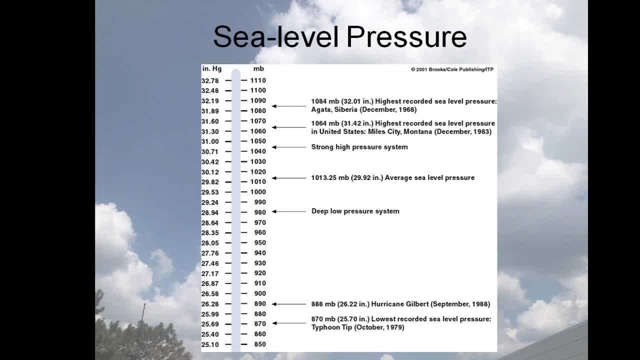 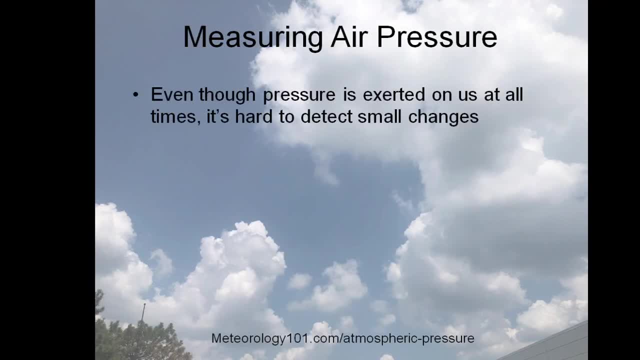 lowest recorded sea level pressure, that's typhoon tip, October of 1979. even though pressure is exerted on all of us at all times, it's hard to detect small air pressure. so if you can, you tell the difference between high and low. do you know how do your aching joints feel? you know? that's where you would be able to. 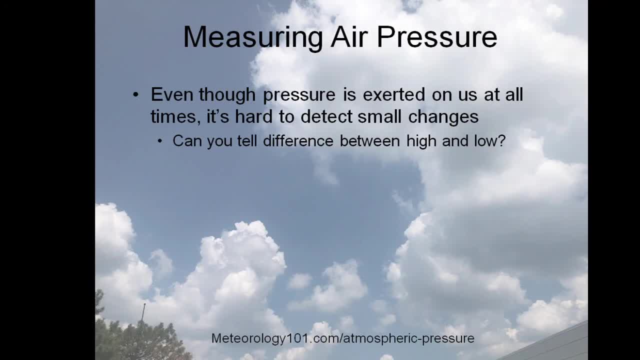 tell the difference. or if you get in an airplane, fly up lower density, your ears pop. you know that's. that's another way to tell. we can detect big changes in pressure like popping of the ears. that's a big change in pressure, not a little change. so 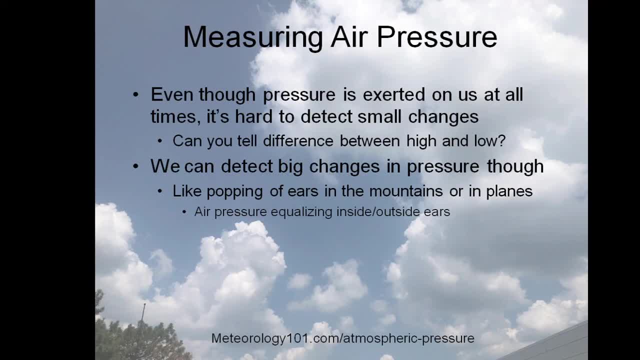 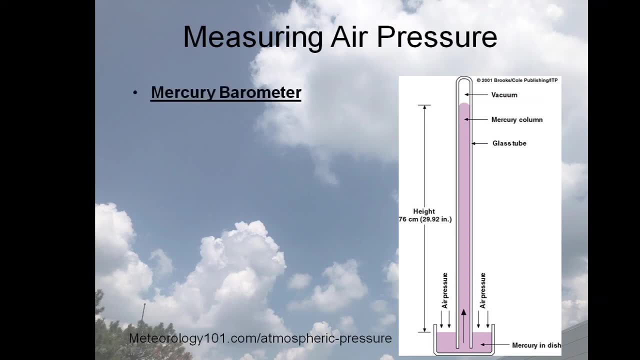 popping of the ears in the mountains or in planes and air pressure equalizing inside and outside of the ears and a mercury barometer. just a large hollow glass tube immersed in mercury so as that pressure is exerted on the outside part of that mercury and the dish it would pushes it up the tube. so that tube. 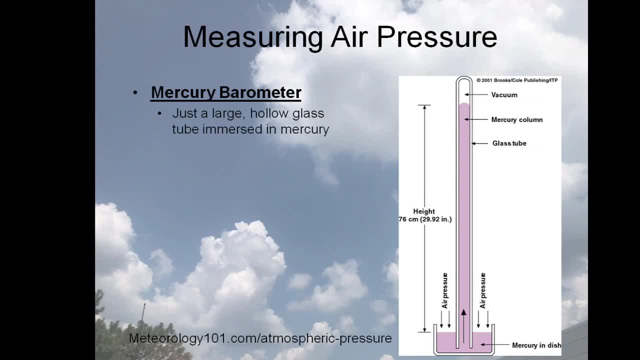 does have a vacuum at the top of that and that empty area. there was a vacuum there because if it had a just atmospheric pressure then it would just build, put more pressure up into that and that liquid would never increase. all right, as air pressure changes, mercury it's forced. 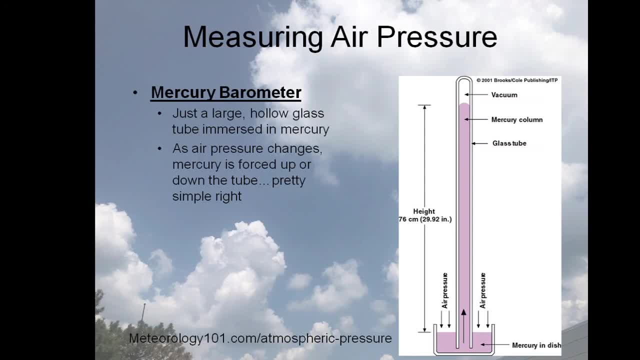 up or down the tube and on average the height of mercury would be 2.99 to 29.9, 2 inches. then that is your average sea level pressure, or thousand thirteen point two, five thousand bars. so typically, if you look at your low pressure systems and 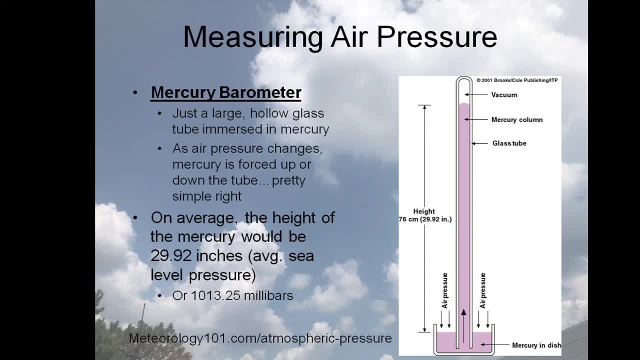 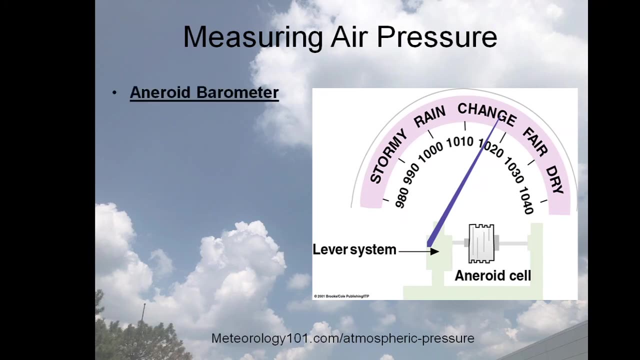 your high pressure systems. anything that is above thousand thirteen millibars is high pressure, anything below that is considered low pressure. and you have an aneroid cell, the lever system. so as this needle moves, pressure increases. then you get drier air, fair weather still. your aneroid barometer is a different style and expands and contracts. 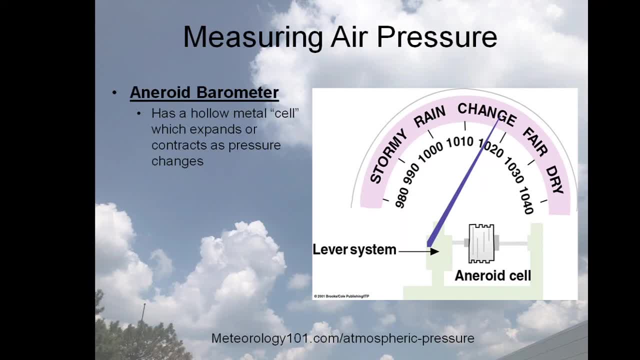 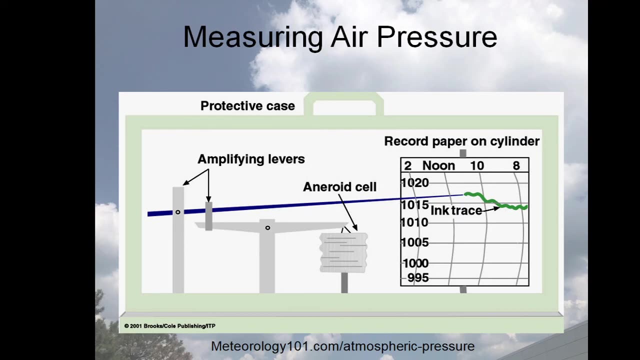 the hollow metal cell which expands or contracts as pressure changes. same type as a three dial weather instruments that people hang on their wall and the measuring air pressure. we're still there, so uh, amplifying levers and our aneroid cell as that exp expands. then this is a roll of paper that 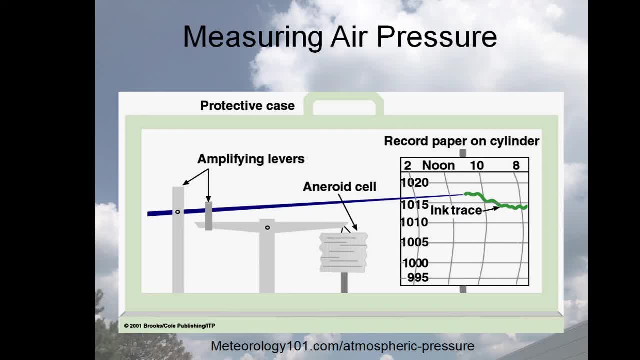 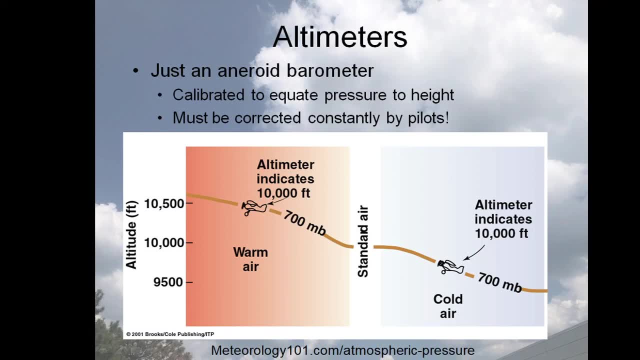 rolls around and the ink draws the line and shows an increase or decrease in pressure. and just an aneroid barometer, calibrated, equal pressure and height. now, timitor, that's what. okay, so here's where it gets important with aircraft. so if you're at 700 millibars, you're flying along. 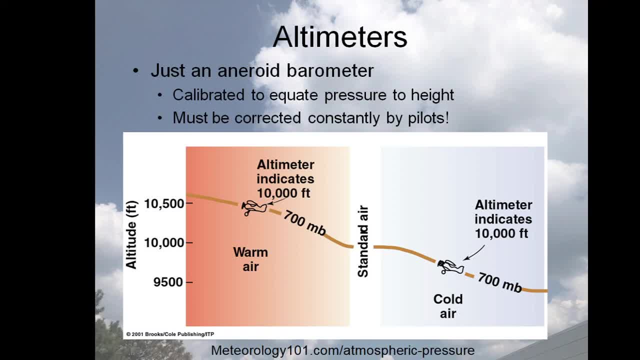 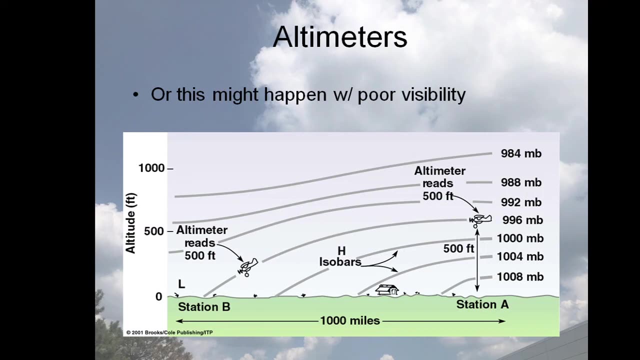 the seven millibar height is rising because you're in a warmer, going into a warmer column of air. they're still reading the same pressure, but they're actually climbing if they so they have to correct for that constantly. so the worst of it would be is if they were going into cooler air, lower heights. they followed a 500. 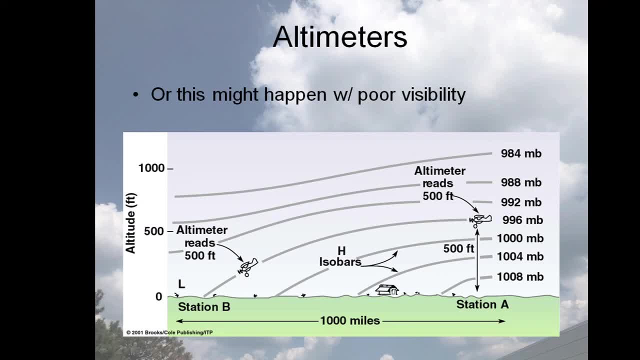 millibar. you know, like this example, uh 996 millibars. if they followed that level and stayed at that level, it actually crashed into the ground because the they'd be going to a surface low and realize it. that's why, back uh years ago, when uh early aircraft with these uh altimeters, people 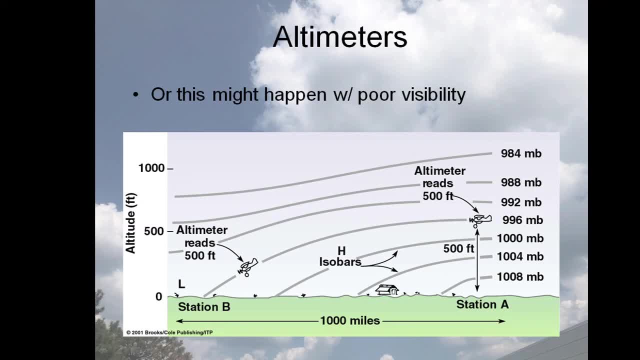 weren't. they didn't understand that, so they were. when those planes would fly through the mountains, they'd actually be crashing into the mountains because they they thought they were higher than they actually were and, of course, poor visibility. so you get into a storm over a mountain, you know. 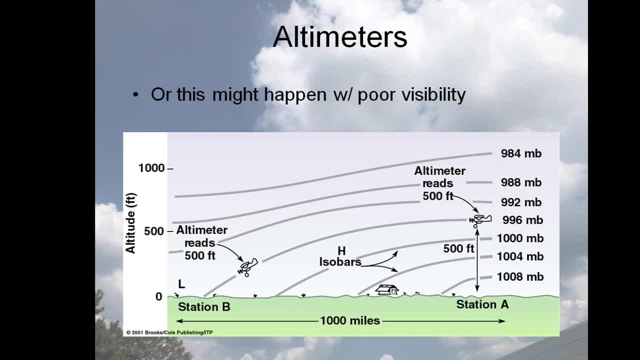 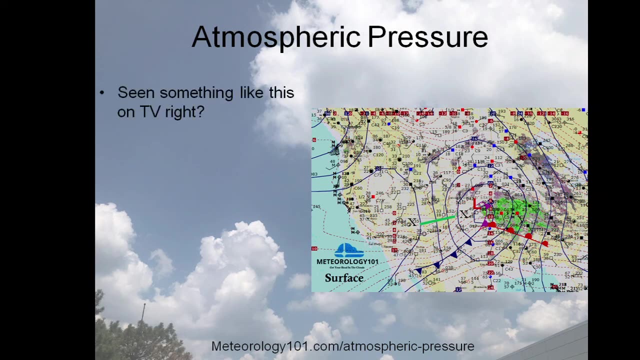 that was the, you know. they couldn't see. they had to go by their altimeter to know what their flight level was, but they didn't know, they didn't correct for it. so that's when they would get into those bad situations. atmospheric pressure, sometimes seen like this on tv. as far as the you see the low pressure systems moving through. this is a chart. 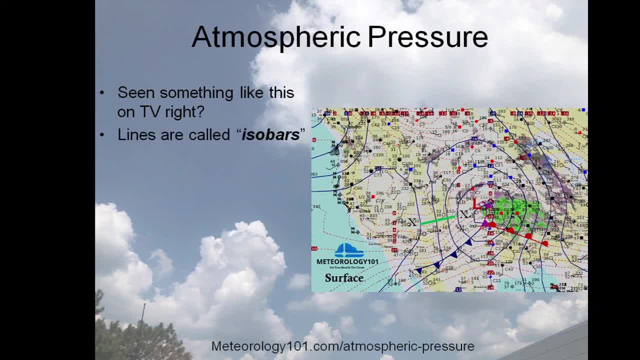 i created and the lines of equal pressure are called isobars and they're measured in millibars. so if the elevation varies across the united states- and it does, and we know pressure challenges quickly with height, then what are these types of maps? all nice and neat. so basically you know. 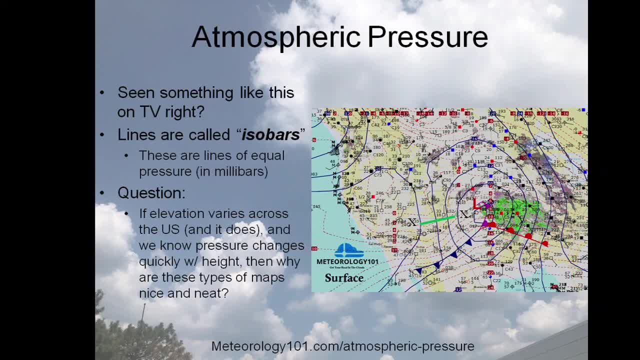 if you actually a lot of the forecast models you look at today, you'll see the isobars and they're all just look like scribbly lines everywhere. it's hard to track them. really it's actually the actual pressure. they're not correct. but if they're not correct you're really. 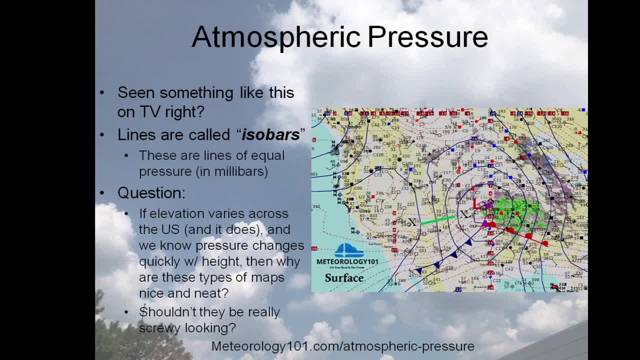 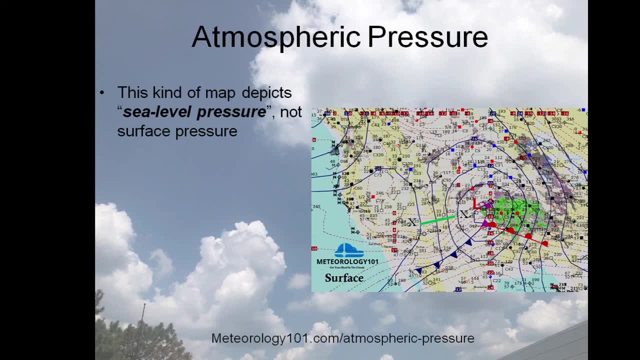 for the sea level pressure. so shouldn't they be all screwy looking so? so this kind of map depicts sea level pressure, not surface pressure. so those are saying they have to be corrected for the sea level pressure because of different elevations. you got a, you got to take that pressure. 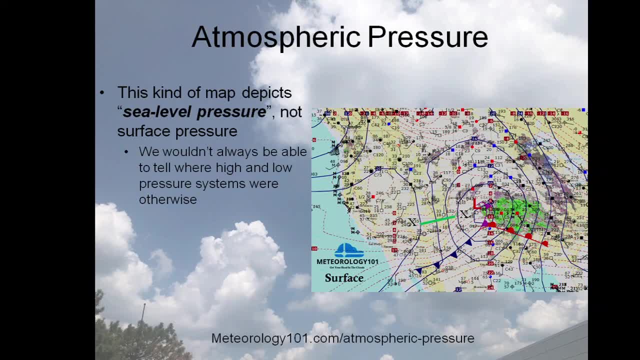 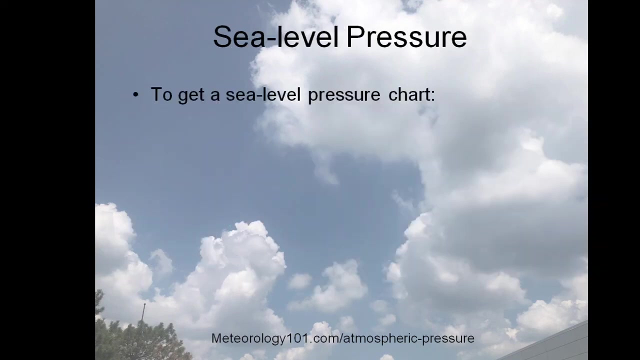 away to change it to depict the sea level, so we wouldn't always be able to tell where the high and low pressure systems were otherwise. if you didn't correct for that, so how do you? we figure out sea level? pressure is at each location where the measurements are taken to get sea. 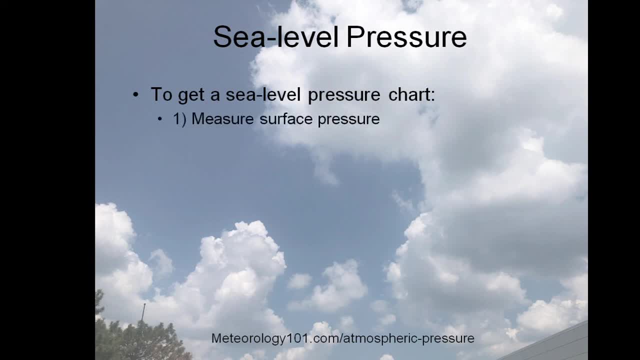 level pressure chart, measure surface pressure and correct for instrument error, temperature, gravity, materials of the barometer and then correct for altitude. so now, when you correct for that altitude, that is where every weather station has a. you know what's their height above sea level. that's where they have to make that. 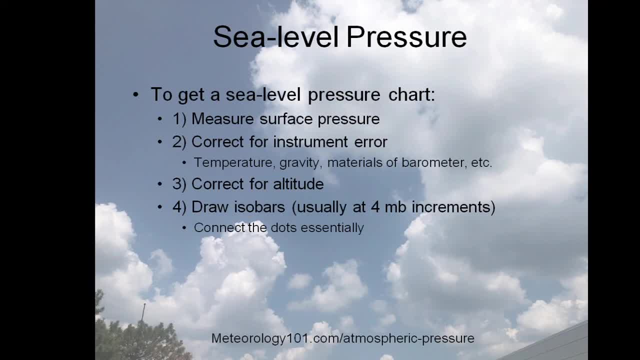 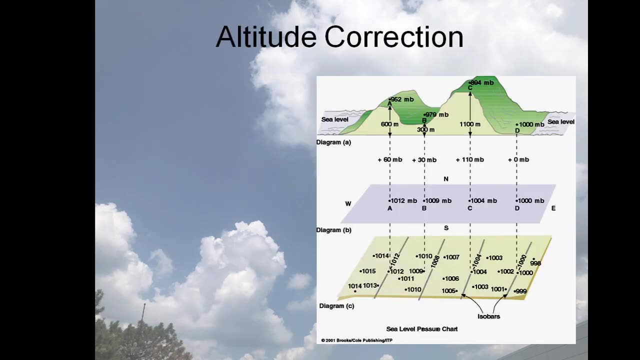 correction. then draw isobars, usually four millibar increments, and basically connect the dots. so one and two are easy. what about three and four? so three got a correct for altitude. okay, so near the surface the earth surface pressure changes 10 millibars per hundred meters. so if a station is 300 meters altitude in 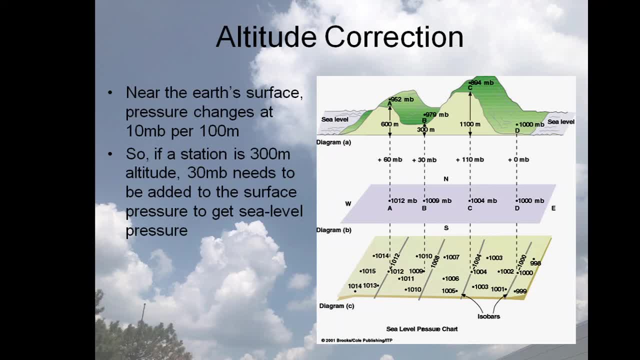 altitude, 30 millimeter millibars needs to be added to the surface pressure to get the sea level pressure. and once the altitude correction is done everywhere, then we can draw the isobars. so if you look at this chart, you have a station, say station a, versus b, and then station c. now you have 1100 meters and on. 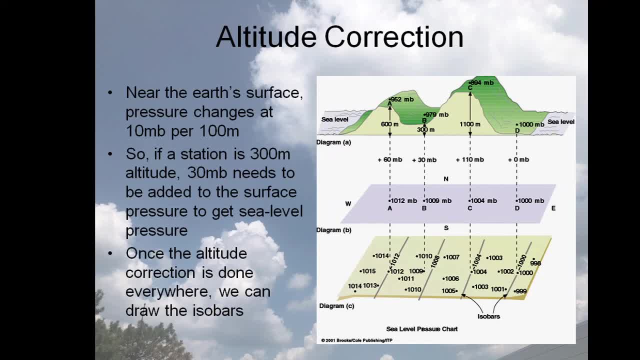 c in elevation, you have 600 meters on station a and only 300 meters on station b. so now you have to minus that 30 millibars at 60 millibars, 1100 millibars, and then there are 110 millibars and then you can drop that down. that brings you to your sea. 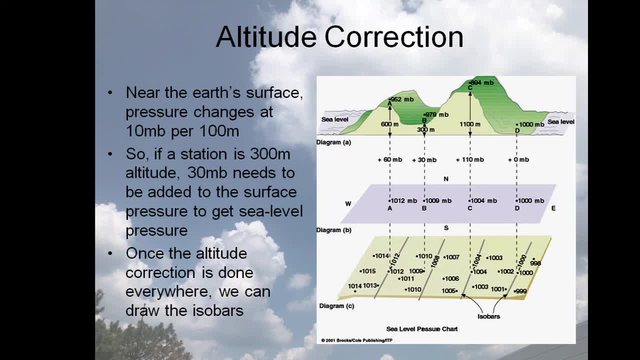 level pressure, and now you have your corrective pressure that is put on the chart and then you can draw those lines of equal pressure. so that's basically: the computers do that for us now, so we don't have to know the elevation of every weather station out there and basically the reasons you do all this. 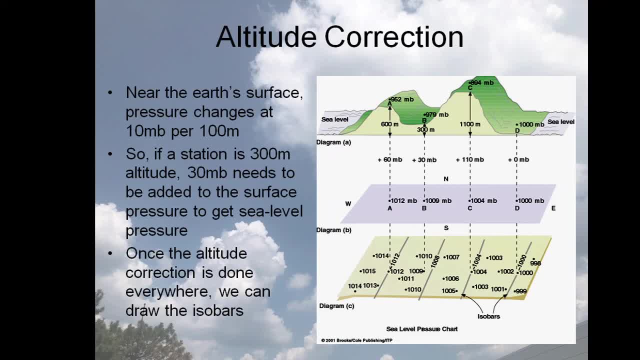 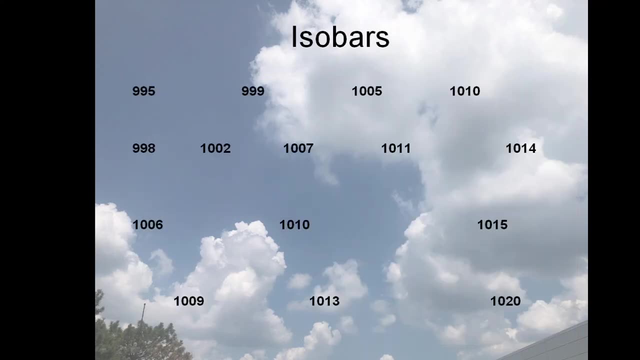 the want to get your surface chart but the there's only so many weather stations out there that let off radio sounds to get the upper air pressures to bring those lines of equal height on the contours. so your ISO bars, these are your different pressures, so we draw a line of equal pressure to get, or basically our system. so 996 we do. 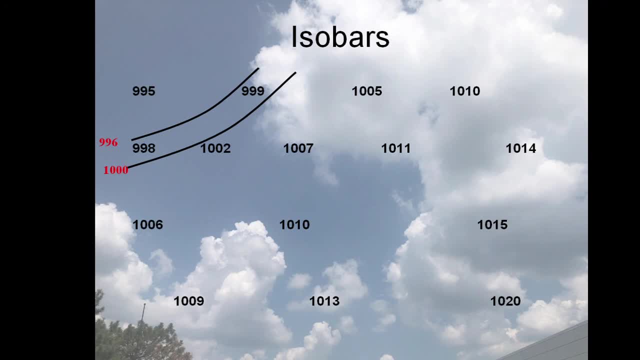 pretty much every four millibars there's a thousand thousand, four thousand and eight, twelve and sixteen. so now you can see where your lines of equal pressure are on the surface chart and obviously this is a like that: 995. that's your low pressure center. and then you 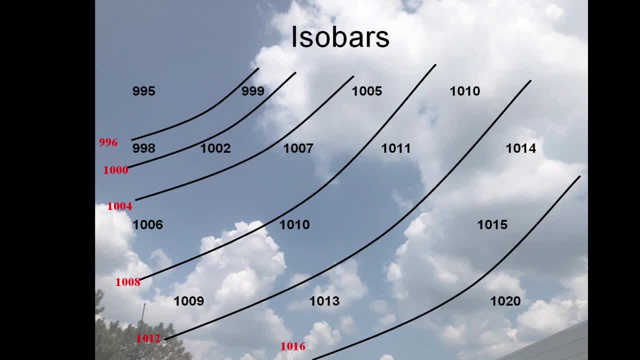 have the tighter ISO bars are closer together and then they start to spread out as you get away from that, that system which is pretty typical: tighter low-pressure system, stronger winds toward that low high pressures rushing in to the low pressure, and you have this tighter ISO bars, that toward the center. 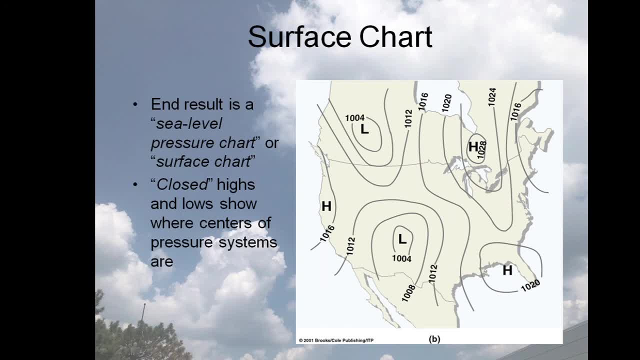 of that low. so the end result is: see level pressure chart or surface chart. closed highs and lows show where the center of the pressure systems are, and you don't always see a closed highs and lows on the surface either. you can just see a trough. so if you just see, 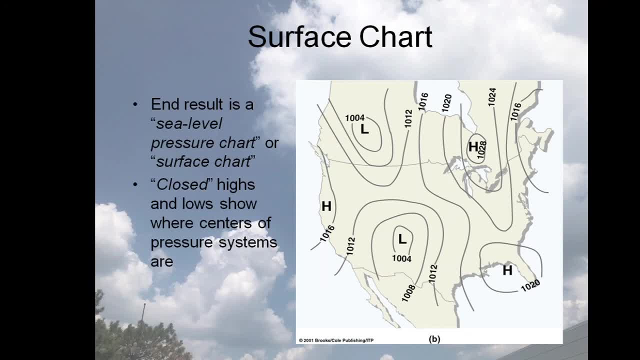 that trough. get rid of that low with the thousand four the top right there over Canada, thousand four millibar level low. get rid of the low, the circle thousand four millibar. now you have a trough and sometimes you can put a look up here. we'll put a L to indicate that's lower pressure, you know, but you can pretty. 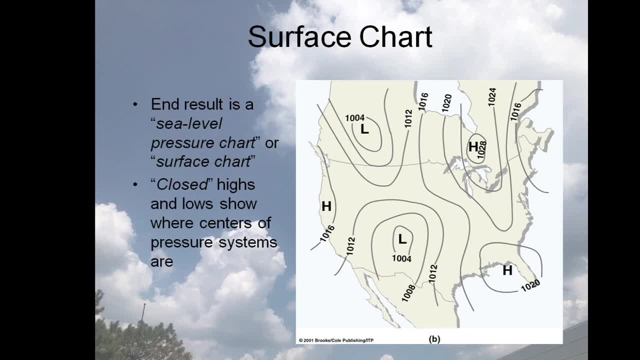 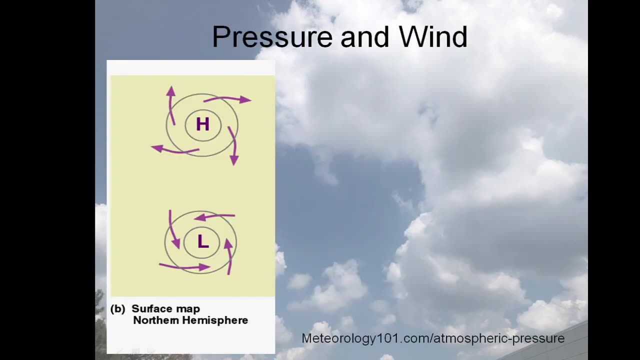 much determine that by the troughing, but you won't always see a closed low, unless that, until that system actually develops, these are all your closed lows and highs. so in the northern hemisphere surface winds blow clockwise and outward from the high pressure, anticyclones counterclockwise and inward around low pressure systems and they're called 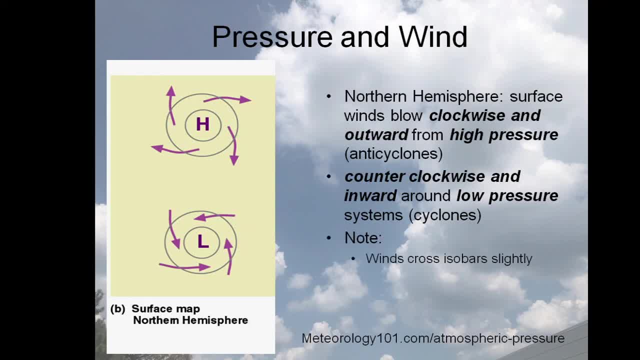 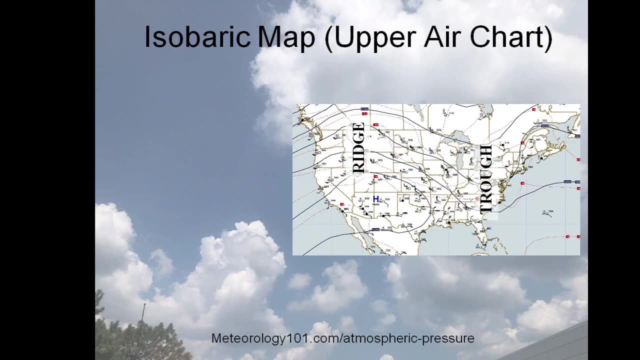 cyclones and winds cross isobars slightly tightly packed. the stronger the winds- so we were saying in the previous slide was closer the isobars together, the stronger the winds are. reverse flow in the southern hemisphere. so if you're ever looking at weather in the southern hemisphere around, 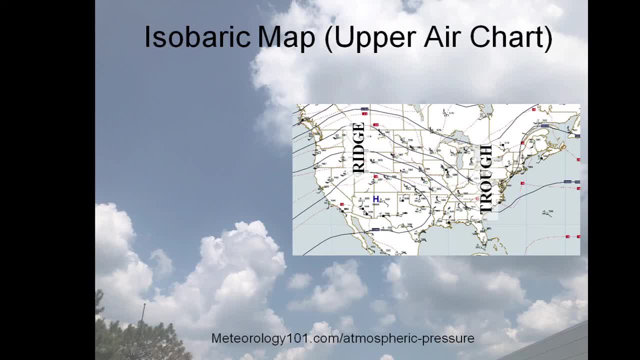 Australia or something, then you have to keep that in mind, that if you're looking that winds flowing around a pressure system, you don't flow the same way as the northern hemisphere, so need to pay attention to that so you know you're looking at a high or low pressure system. 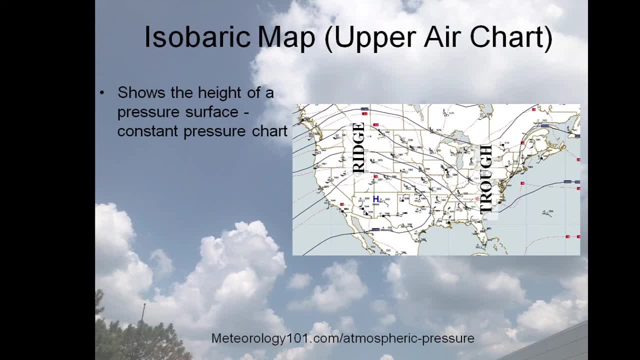 iceberg pageant upper air charts. okay, these upper air charts are lines of equal height and having about 100 centimeters of an kansard's algorithm. and then you have the point here, the ldUT, and then height. there are contours to show the height of the pressure surface. 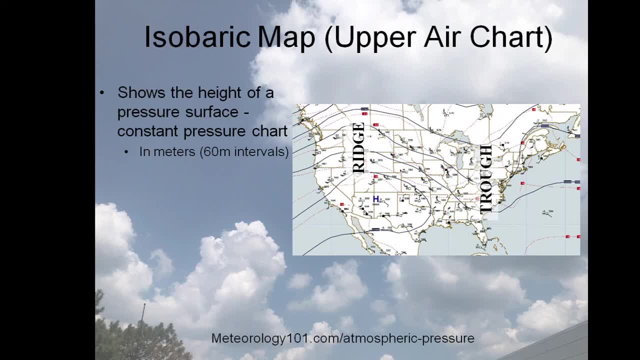 and they are done in meters, 60, 60 meter intervals, and this one is the 500 millibar level. all right, so pressures, surfaces are higher up in warm air, so it was a higher warm air. a warm air column expands and goes higher into the atmosphere. 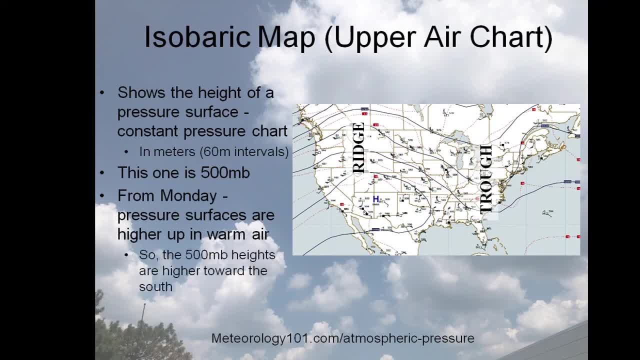 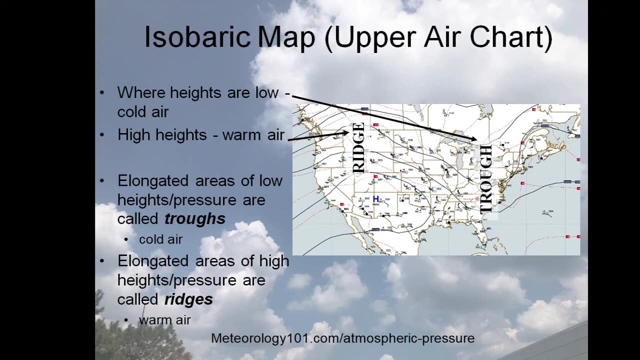 so over a warm column of area of higher heights. so the 500 millibar heights is higher toward the south. this warmer in the south, colder in the north. so your 500 millibar level is higher at this in the southern part of the united states, toward the equator. so 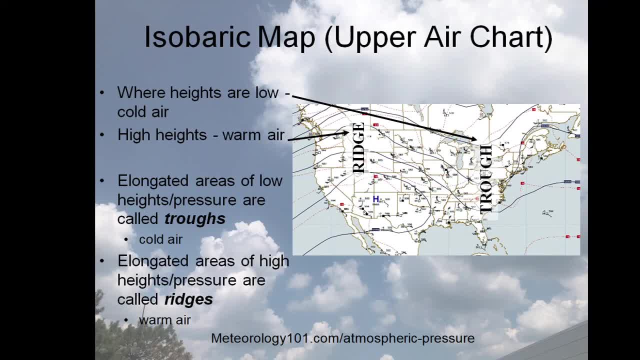 that's where it's located. where heights are low, there's cold air, so that's through troughing and high heights is warm air. elongated areas of low heights or pressure are called troughs, that's cold air, and elongated high areas of high pressure, of high heights or pressure are called ridges, and that is warm air. 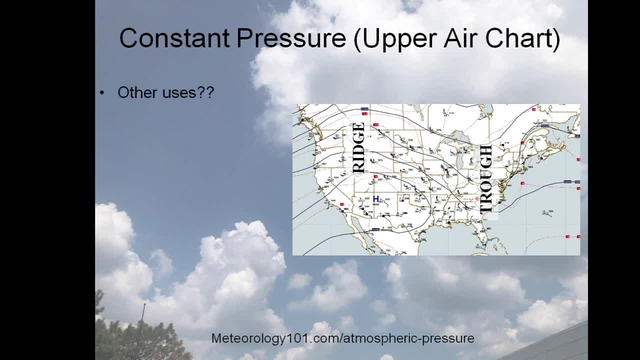 and constant pressure, upper air charge. other uses: wind shows us direction and speed and, like the surface map, except for winds, tend to blow parallel to the height lines. so on the surface you have friction and actually friction will cause the winds to slow and back and they won't blow parallel with the iso bars. in the upper levels you have 11 3.9. 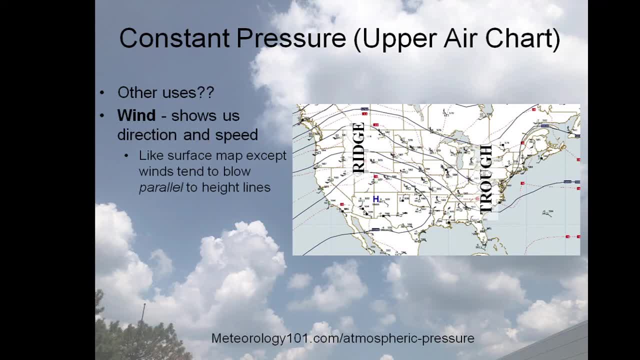 friction, so the winds will blow more parallel with the contours. closer the lines are the same thing, the higher the wind speeds and steering upper level winds determine where just surface systems go and whether or not they strengthen. so now you're looking at typically, if you look at a low pressure, 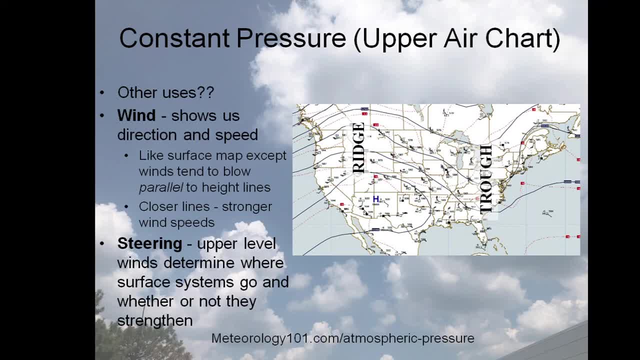 system moving through the United States, you want to know how fast that system is moving. or even the cold front. look at the winds behind the cold front. your typical rule of thumb on that is 50% of the 500 millibar winds. so if you had a 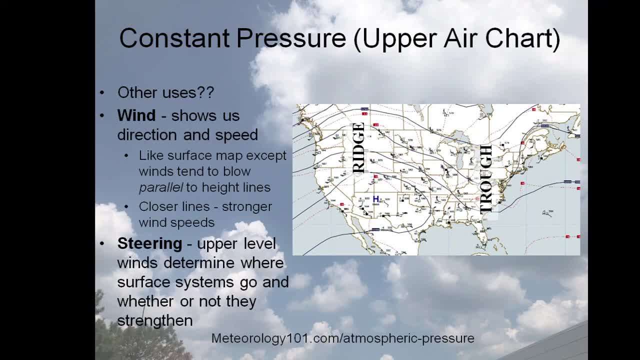 500 millibar wind of 50 knots and that system or that front is. the rule of thumb is that it's moving at 25 knots and 700 millibar level is 70% of 700 millibar level winds and you'll notice as you go up in the atmosphere that went the stronger. 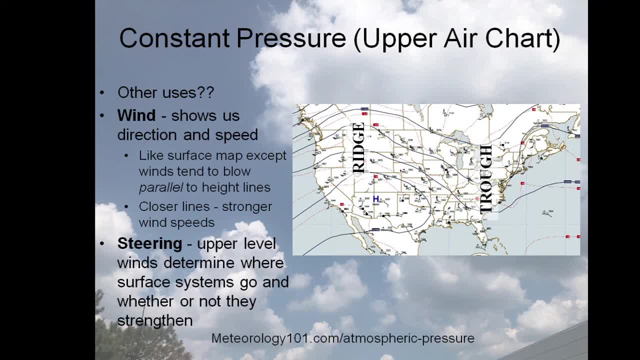 the winds are. so the typical rule of thumb for upper level winds determining where the systems go. if you look at the troffling and the bridging that is, your steering flow in the upper levels now the speed of the systems is typically. if you look at the, where the 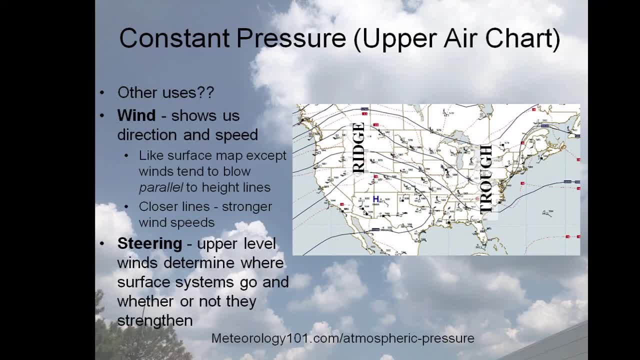 surface front is, and then you pull up the 500 millibar chart or the 700 millibar chart. 50% of those winds at the 500 millibar level is going to be the speed of that system. how fast that is moving. 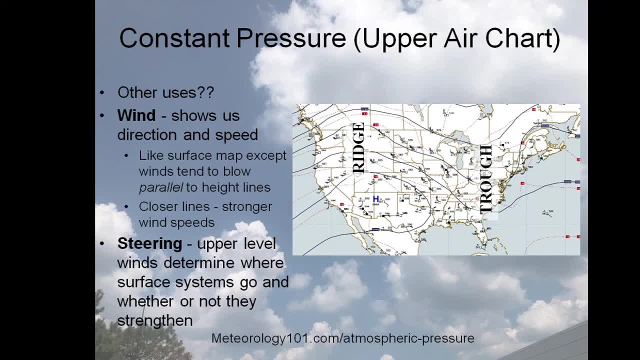 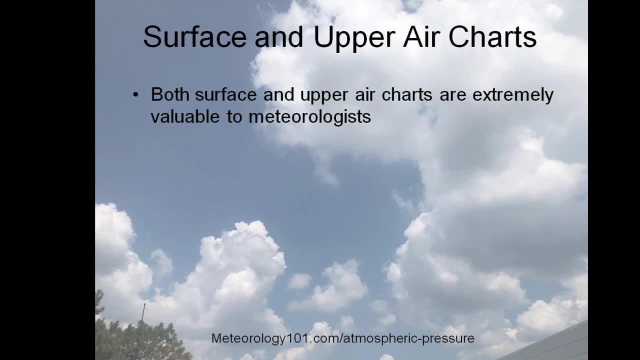 And the 700 millibar chart is 70% of those wind speeds. That's going to give you an average, just kind of a rule of thumb, for how fast that system is moving. All right, so both surface and upper air charge are extremely valuable to meteorologists. 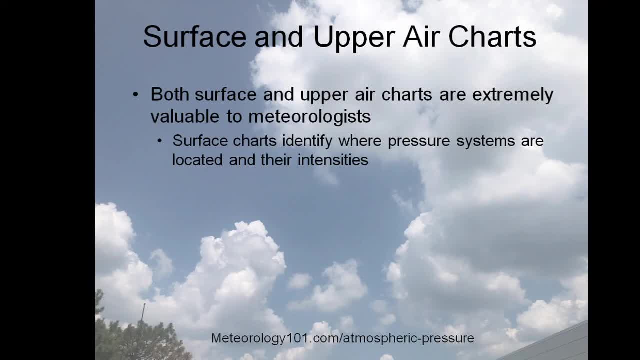 Real quick on that. if you look at today, meteorologists actually use the upper air charge to determine the strength of these systems. A lot of the guys you see on YouTube are just models, readers, interpreters, that's all they are. 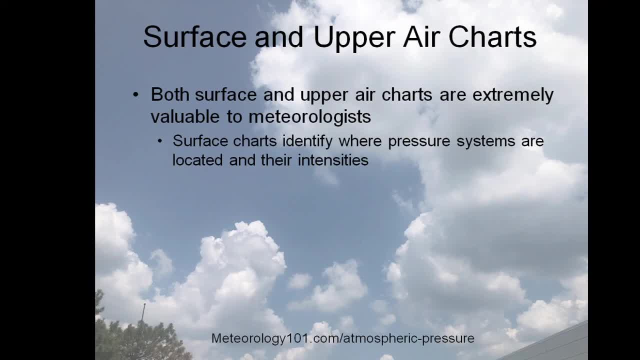 They're not forecasters. They just kind of look at the models, say, hey, there's the moisture that the model's depicting. You've got to understand the upper levels and how intense these systems are going to be. The models may not pick it up. 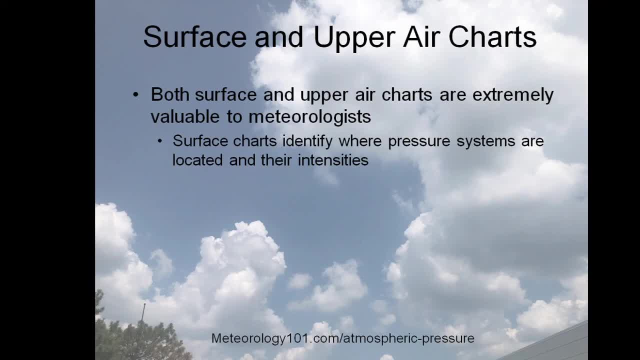 So, going by what those guys say, they all got disclaimers that they're not forecasters and it's for entertainment purposes only. So I'm glad they do that. But if you look at their forecast models, you've got to understand the upper levels. 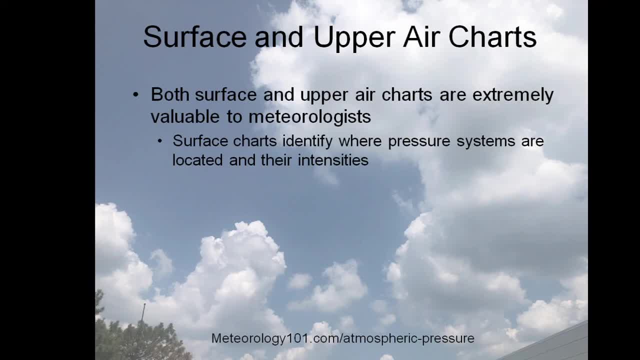 to understand these systems. If they're going to fill, they're going to fill. If they're going to fill, they're going to fill. If they're going to fill, they're going to build, they're going to deepen, you know. 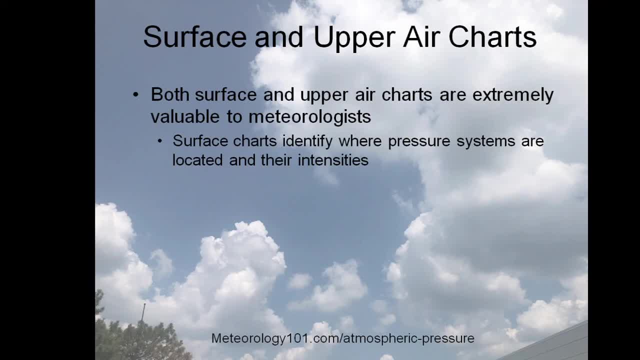 high pressure's going to build, you know, or weaken, then you're going to be. you know that's where you're going to find out how much of that system's actually affecting something. you know You'll have meteorologists, even meteorologists at weather stations. you know they'll tell. 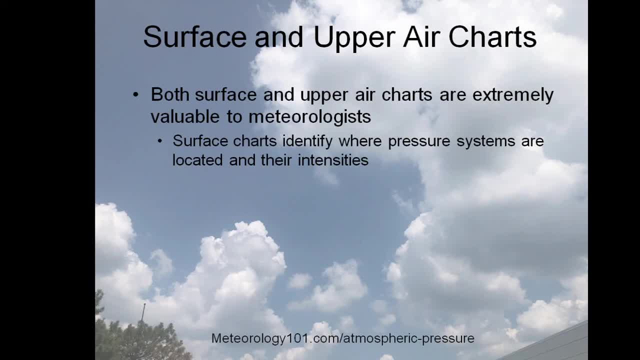 you all this snow's coming and all of a sudden you get nothing. Or they'll tell you you're only going to get 1 to 2 inches. the next thing you know you'll get 5 or 6.. So I mean, you know that stuff's hard to determine. 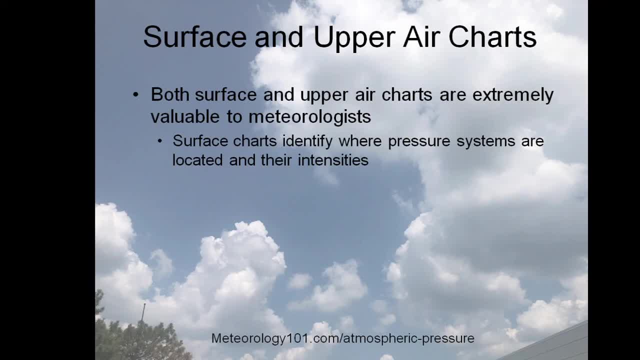 Basically, they are going to click off the forecast models. That's good. If they were going to slow you down for a short time, you'd be asking for extra funds. And if they were going to say, hey, don't Anda promise federal payments, and you'd be. 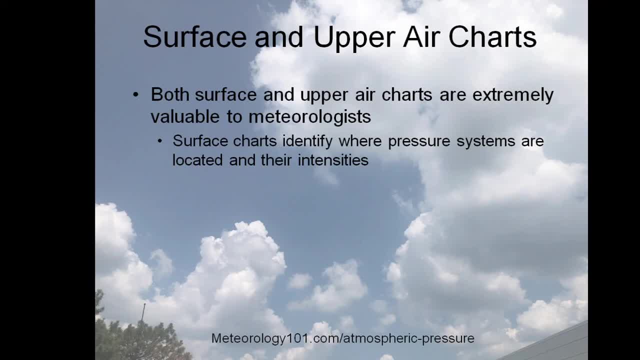 models for that. so, but you have to be able to verify those models off the off of these charts- the surface and upper air charts. that's actual data that you have to verify those models against to make sure they're handling that system properly and then to determine if they're actually going to forecast that. 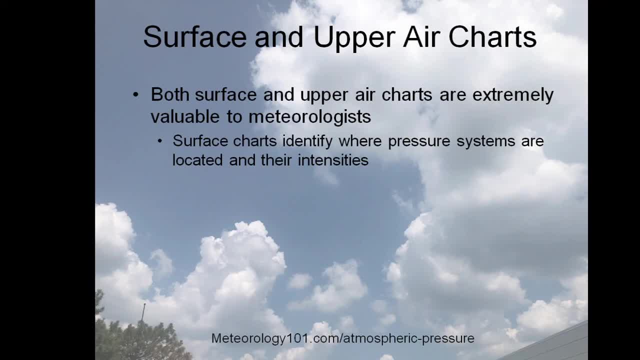 system correctly alright. so service charts identify where pressure systems are located and their intensities. I mean upper air charts indicate where these systems will move and how they will strengthen and weaken in time. I mean that's true, and but also the upper air charts is the that's going to? 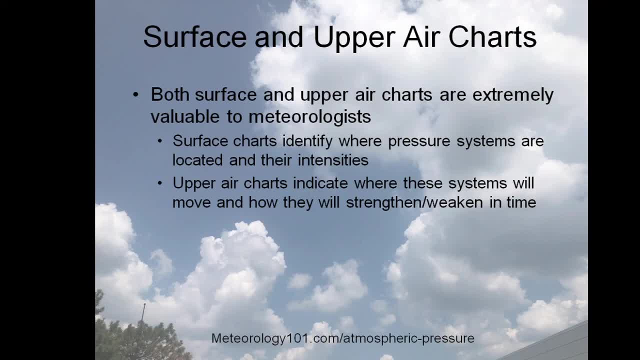 determine the intensities also. so don't forget that part. I mean you can look at the intensities on the surface. yeah, that's your low pressure system, the 998 millibar. you know. low pressure system, you know, and it's deepening as it moves. but if you don't know what the upper air, the levels are doing, you know. 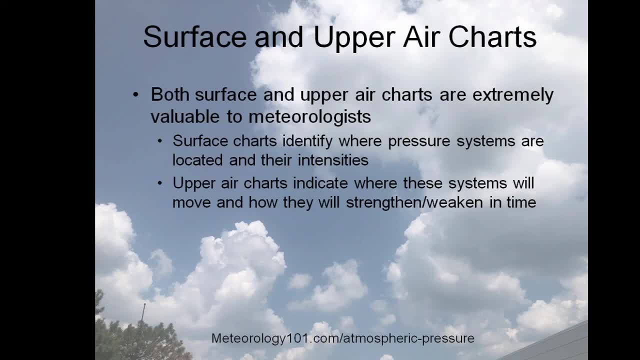 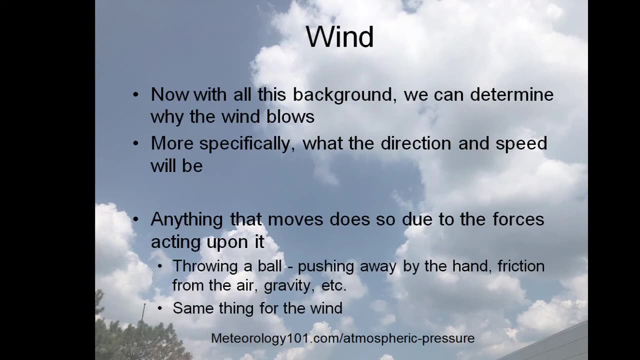 the overall impact of that system. nothing could fill you know overnight. next thing you know, you know the low pressure system is gone. so upper air for intensity is a is a big deal. so with all this background we can now determine why the wind blows. I guess I got a little off topic there. this video is for pressure and wind, so 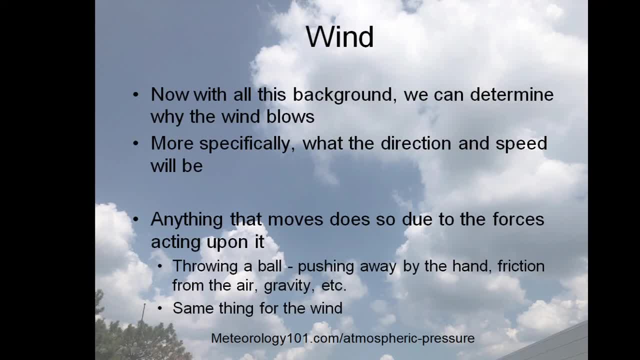 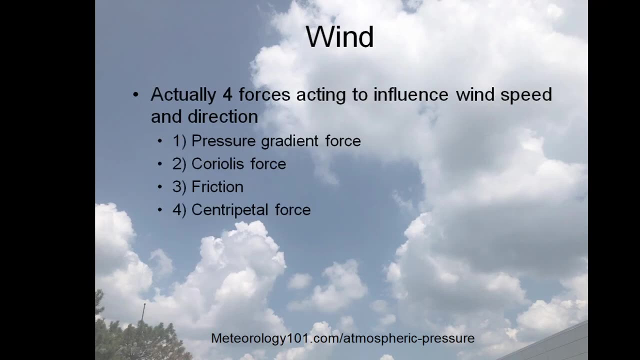 more specifically, what direction and speed will be? anything that moves does so do the forces acting upon it. so throwing a ball, pushing away by the hand, friction of the air, gravity, etc. same thing for the wind. so for actually four forces acting to influence wind speed and direction: pressure gradient force. the stronger the pressure gradient force. 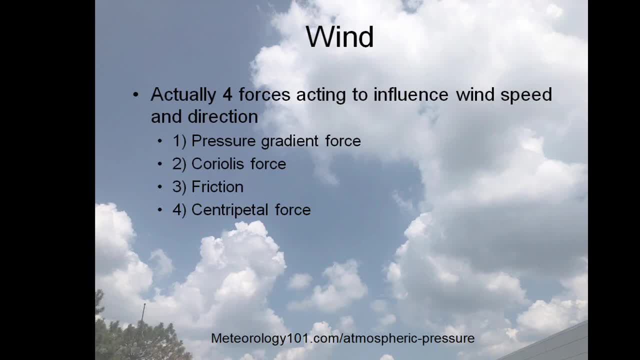 the stronger the wind is. that's your pressure. gradient forces to how far apart are those isobars spaced and that's going to help you determine the wind speed. Coriolis force- that is the rotation of the earth. so now you're going to have another outside force impacting that air parcel. that's moving. 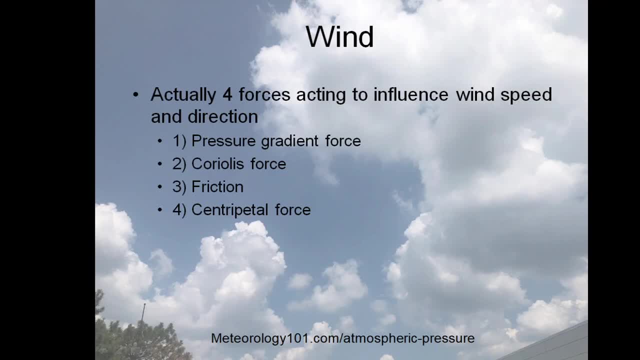 and that's how that direction is going to actually change: from the Coriolis force and then friction. you know I did mention earlier the friction is will slow and back winds. so your direction and your speed changes from friction and centripetal force, that is, the force going in toward the center of an object. 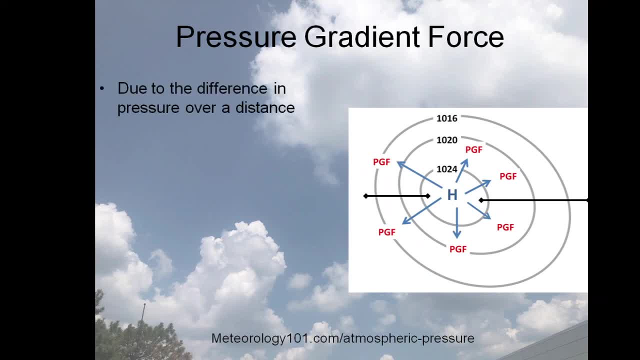 so pressure gradient force. due to the difference in pressure over a distance, the greater the pressure gradients lead to a greater pressure gradient force, and hurricanes are a good example. very low pressures in the center. pressures increase rapidly as you move away from the center and you have a strong pressure gradient force always. 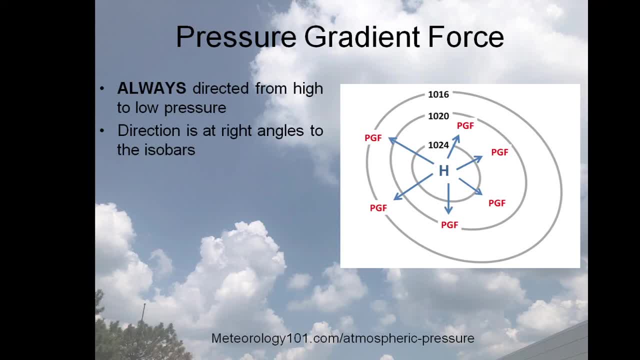 directed from high to low pressure. high pressure always rules high pressure. a low pressure system, even a hurricane, being a low pressure system, goes and smashes into a high pressure system. the high pressure system doesn't move the low pressure system, the hurricane, even it's so intense, it moves around the high. 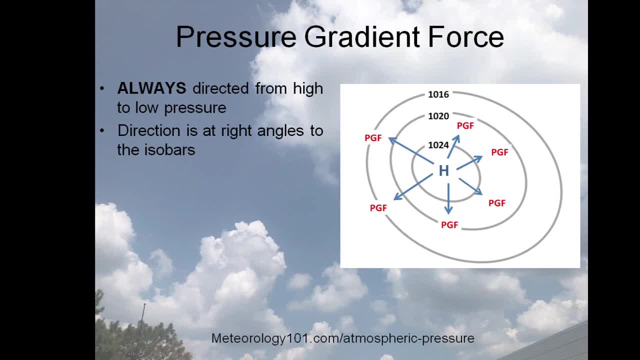 pressure system. it will never move. that high pressure system direction is at right angles to the ISO bars. so your pressure gradient forces out from a high in toward a low. and it is at a right angle, 90 degree angle to the isobar. so what does that mean when the wind blows? 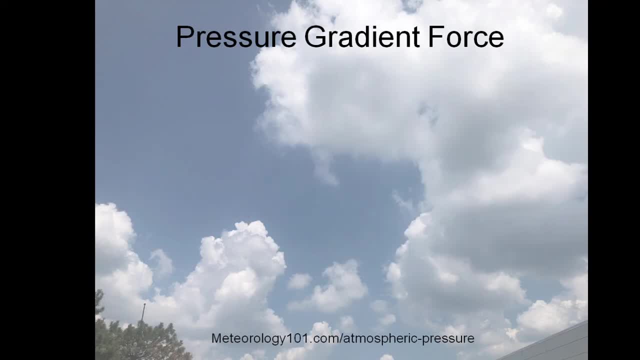 directly from high to low and now you have the other forces. so since pressure changes much faster from high, then with height, then horizontally isn't pressure gradient force strong in the vertical. so now if you decrease what height pressure decreases with height, then basically your pressure should be shooting up vertically constantly. but 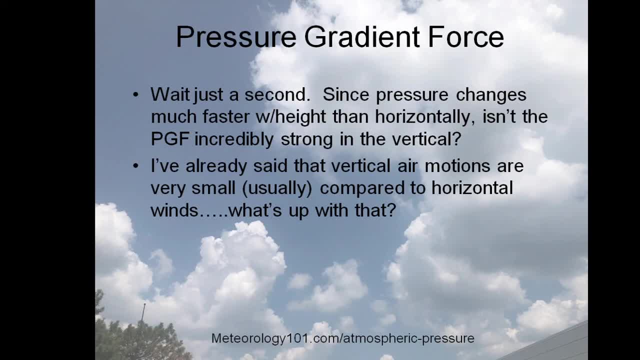 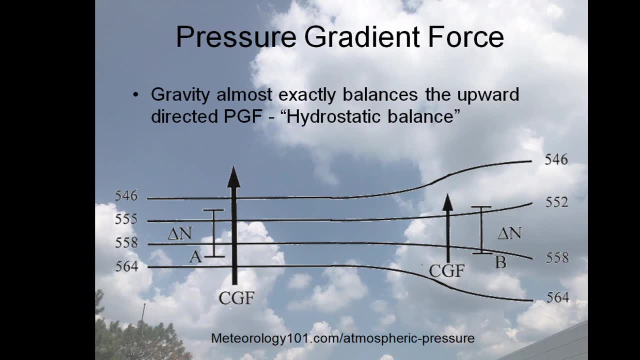 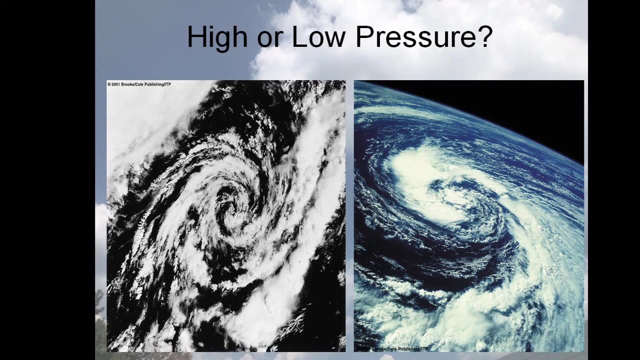 we already said that vertical air motions are very small usually compared to horizontal winds and if you look at that, gravity has an impact that wind can't blow up because gravity is pushing back down on. it almost balances that out to hydrostatic balance. so how do you determine if you have a low? 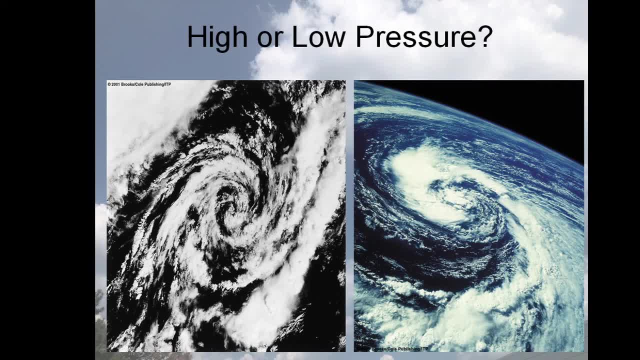 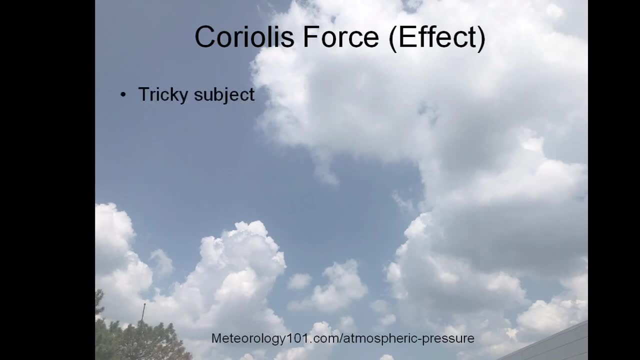 higher, low pressure. look at the circulation in these pictures. there is high pressure and there's your low pressure. then accordingly, all it's a force force. okay, this is a tricky subject just because people, a lot of people, disagree with this force. it's an apparent force due to the rotation of curvature of the 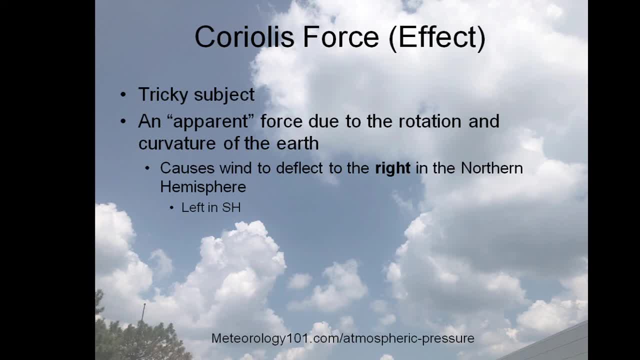 earth causes one to deflect to the right and northern hemisphere and to the left in the set of southern hemisphere, because of that rotation of the earth as the wind blows, then you have a slight curvature as the earth rotates and that will force that right forces at a right angle to the wind. 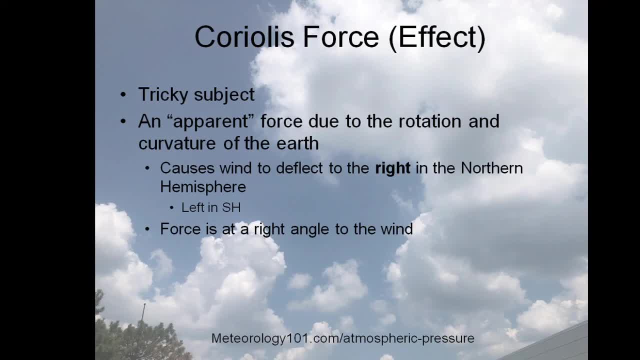 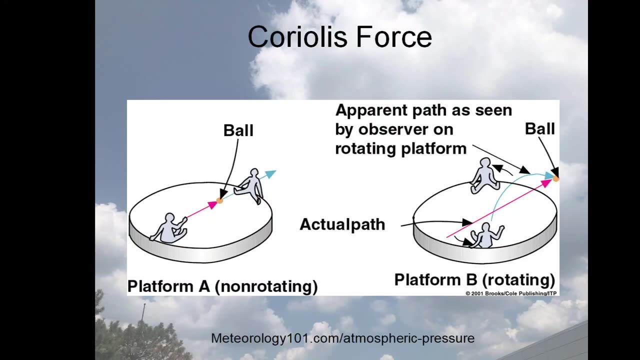 so it is a direct cross impact to that wind direction and things drain differently in the southern hemisphere. so what colloidal is for is if you're sitting on a platform and you're rotating, that it's rotating. you roll that ball to the other person. a non-rotating 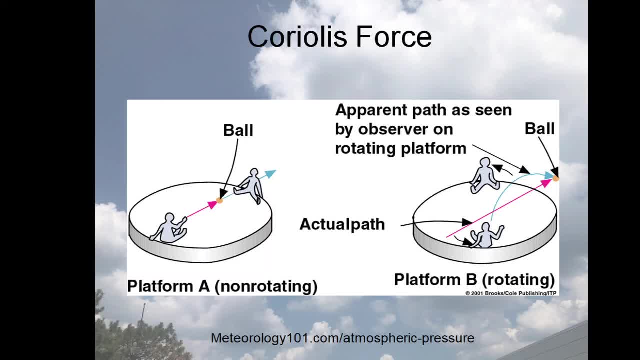 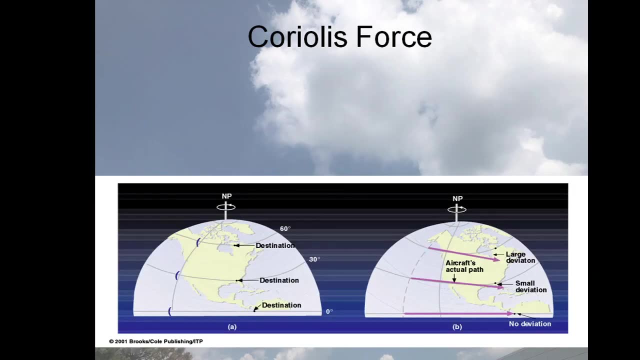 platform it's going to go straight to that person and if you rotate the platform then you roll that ball, then it veers to the right because the rotation of the earth so maximum at the poles and zero at the equator, because basically your wind directions, your winds are very minimal. 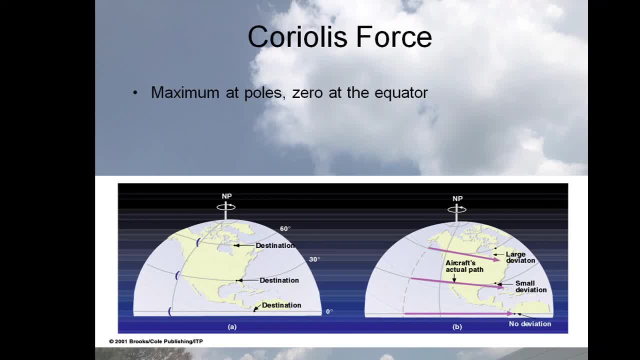 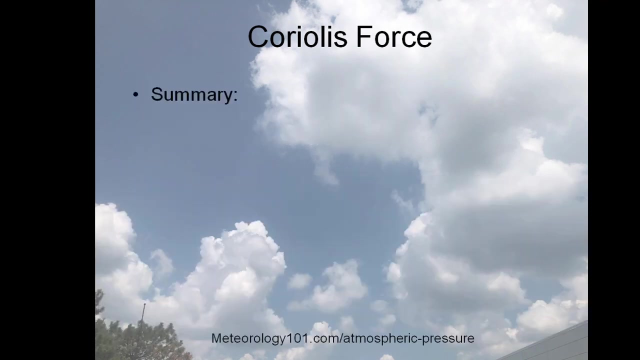 you got your trade winds at the equator, but uh, it's almost, uh, pretty much zero balance, because your, the sun, is at the equator and you got the upward vertical motion: faster speeds, stronger colloidal force, while aircraft fly in circular path. ok so 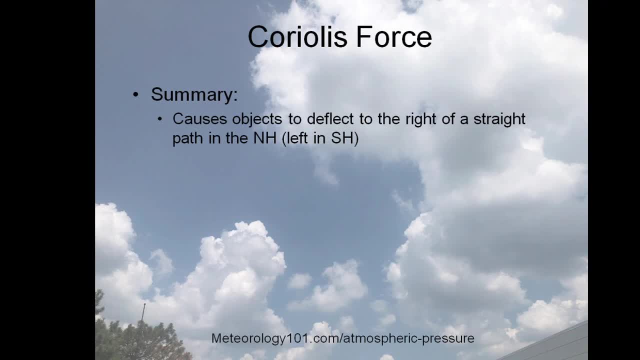 causes objects to deflect to the right of a straight path in the northern hemisphere, left in the southern hemisphere. amount of deflection depends on rotation of the earth, the latitude, speed of the earth, rotation of the form of the earth, which is like the earthup point. 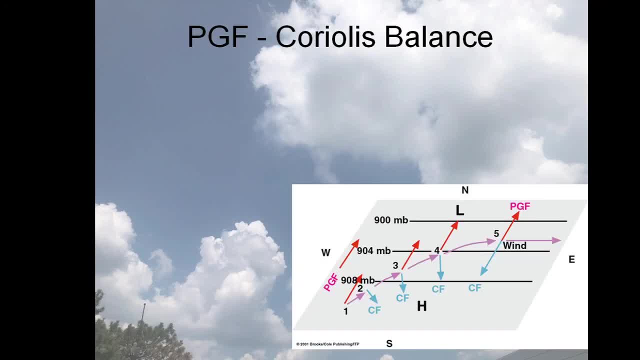 more than some earth Institutes with monitor anymore�. the Wind direction, которая object, the wind, the plane, and then pressure, gradient force and Coriolis force balance. so now, above the friction layer, near the surface, pressure gradient force and Coriolis force roughly balance each other, because you don't have to. 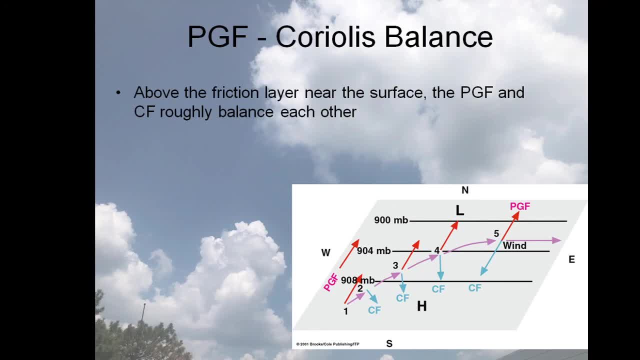 play with. there's no friction at this level where we're above the friction layer. so once friction, that's another force that comes involved if you're actually on the surface. that's why air law flows parallel to the isobars, because you have less friction. wind which flows at the constant speed parallel to evenly spaced isobars is 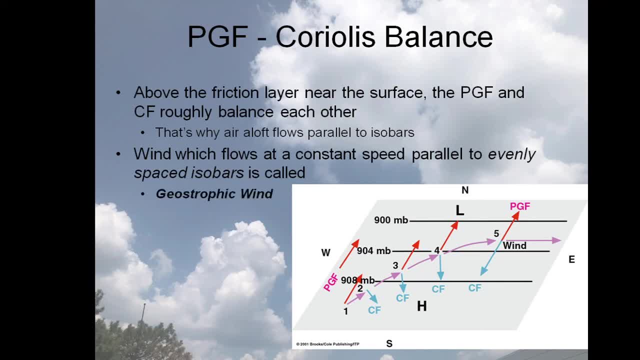 called the geostrophic wind, and there actually is a geostrophic wind scale. should put that in here. it's just your winds flowing parallel to the ice or bars, the spacing of the XRY, so ours, the geostrophic wind scale, will tell you, based on that spacing, how fast, which. 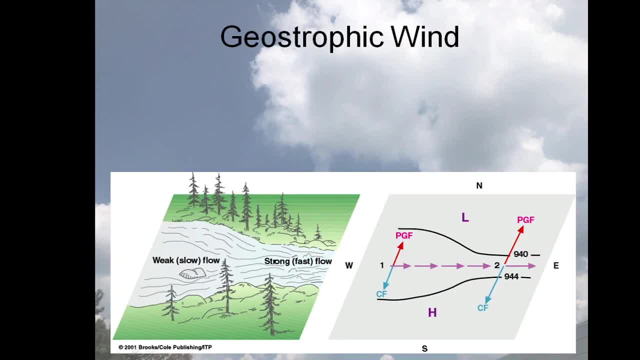 should be what your wind speed should be. there's a scale for that. a lot of meteorologists used to use that until today, as all the technology to day. they don't need all those older charts and tools. always low pressure to the left and then chanting wind, because it's constantly. geosurf Lancer. all this stuff later a lot of geosurfing will tell you, based on showcasing speed, is a replacing the potential of mounting for this small Research. but then, once you get used to it, it's perfect, even better than if you apply the geostrophic까요. 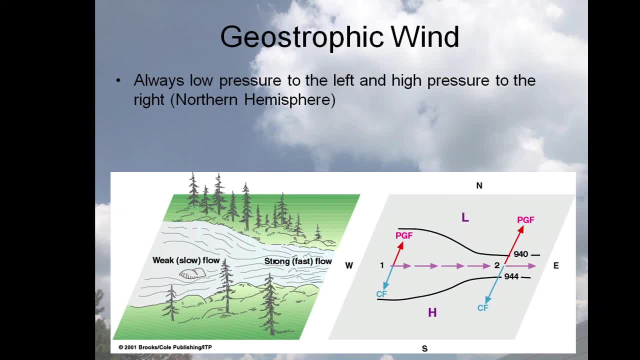 AU can justsky a little into the work so you don't want to be so critical with the and high pressure to the right in the northern hemisphere. so this is basically: uh, come at a second. speed depends on the packing or tightness of the isobars loosely packed with. 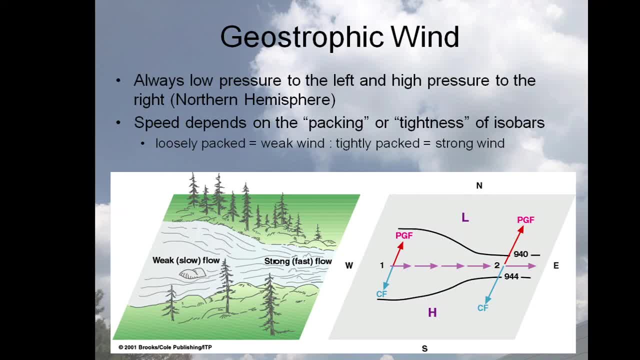 a weak wind, tightly packed with strong wind. so, as we mentioned, the tighter the isobars, the faster the wind speed. but your low pressure to the left and high pressure to the right that this body's balance law is. with the wind to your back, low pressure is always to the left.